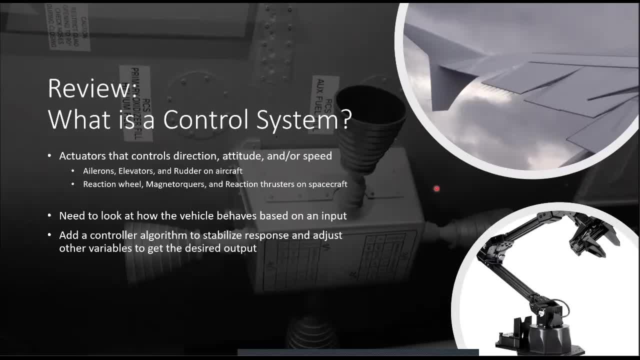 like little puffs of gas, right, That kind of spin the spacecraft around, But like also something like a robot arm that's also a control system, And something like the gas pedal in your car steering wheel, The thermostat in your house, Pretty much anything that takes a human input. and then 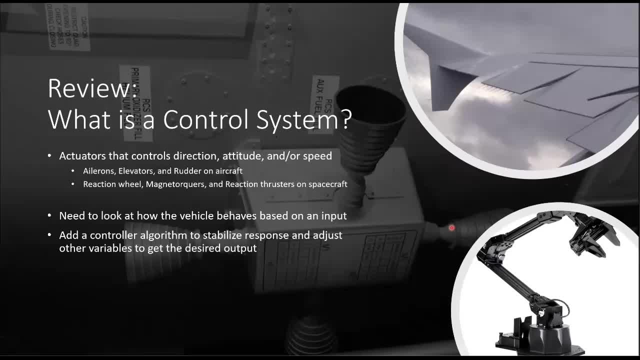 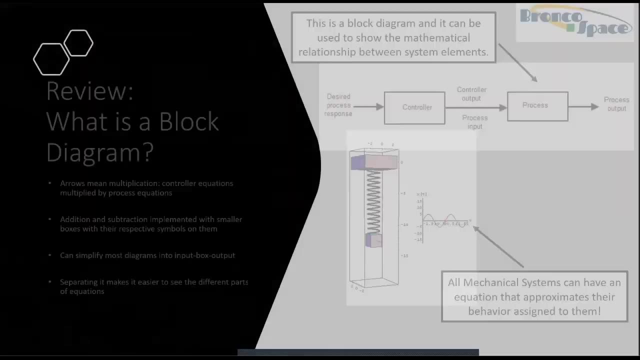 causes a physical change in a physical system can be considered a control system of some sort. On spacecraft, we have three main ones, which are reaction wheels, magnet workers and thrusters, which we'll talk about some more later on. One of the things that is important to understand when you're thinking about control design is also 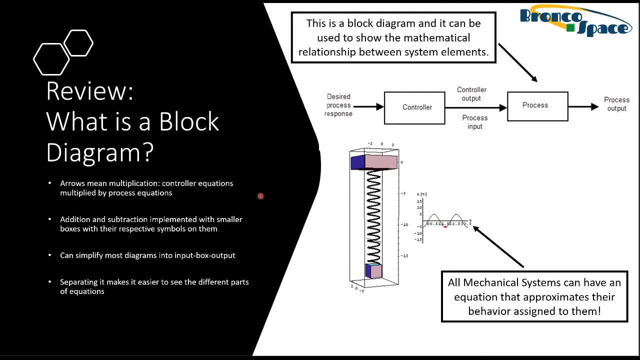 block diagrams, because that's usually how you'll see these systems represented. Now you don't actually need to understand so much for this purpose, like how to do like block diagram, math or anything like that- But when you take your controls class in university, 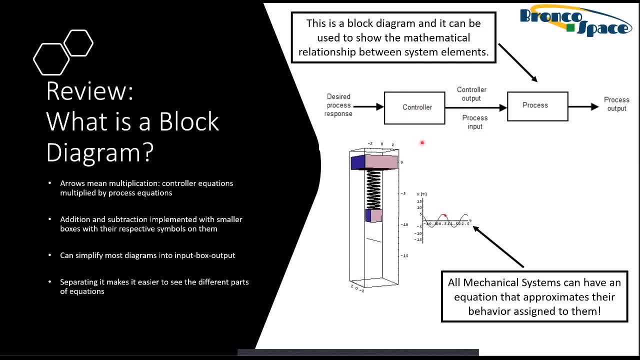 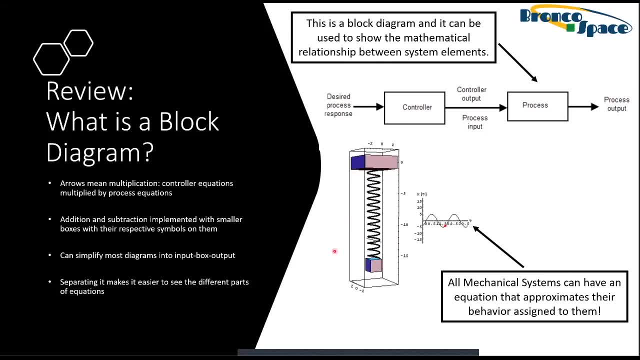 So in this case this mass spring system can be approximated mathematically. In this case this mass spring system can be approximated with a sine or cosine function, because it has a sinusoidal motion. And this is sort of the entire basis of how control systems are, at least. 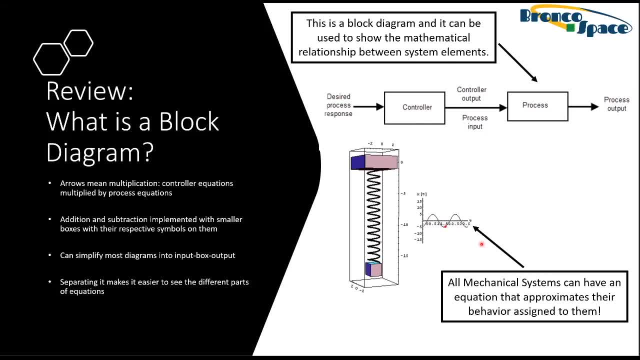 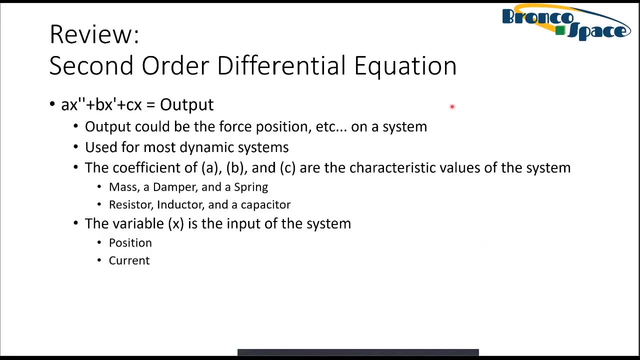 initially designed right. You try to model the system mathematically and then you try to analytically determine what you can change about it to get it to perform the way you want it to perform. So most of the systems that you learn in university you're going to be dealing with. 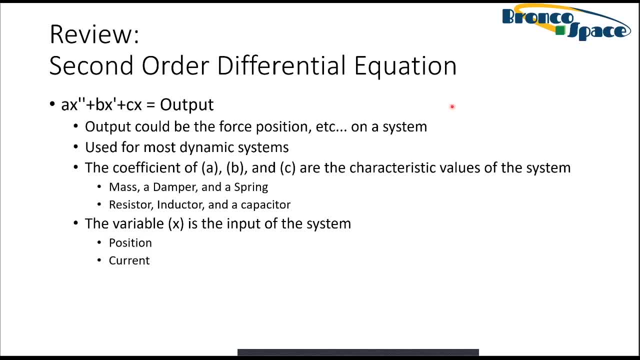 second-order differential equations. Don't worry too much about the math. We're not really going to do math during this presentation, But the important thing to know about second-order ODEs is that they can be solved right, And usually second-order ODE is defined as a system that has 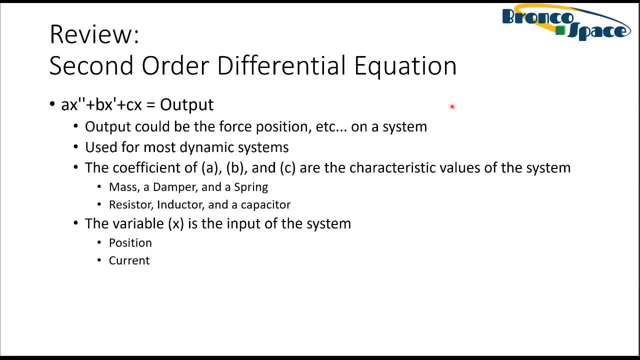 three characteristics about it that change, And they can have less than three characteristics, but if it's more than three, right then you're in trouble because that's a system that actually cannot be analytically solved and there's a lot more complex math as you go into it. 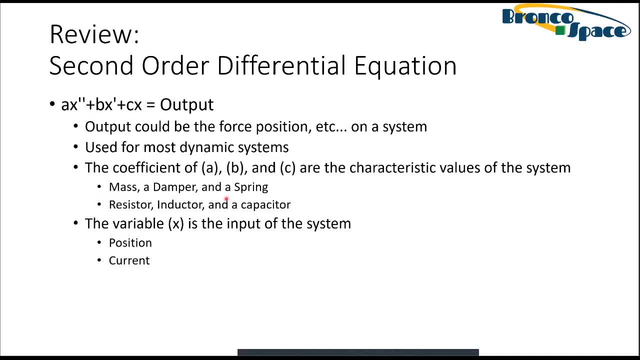 But examples of a second-order system are a mass, a damper and a spring. If you're an EE, something like a resistor, an inductor and a capacitor might be more up your alley. But for the sake of just basic control and satellite, 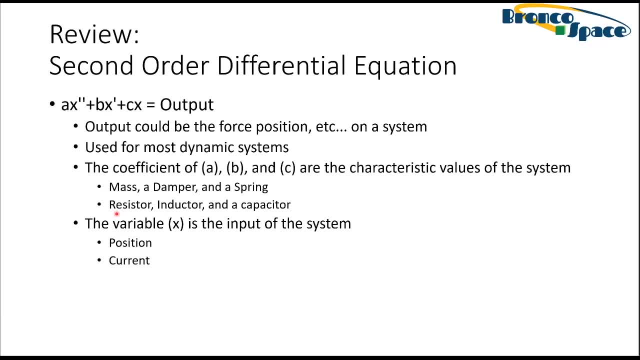 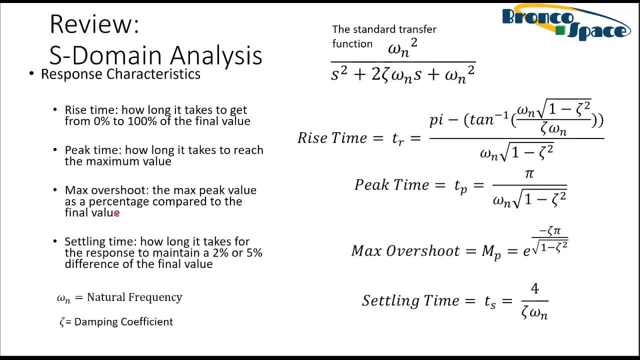 oftentimes you can idealize the system as a mass damper spring system. Yeah, don't worry about the math too much. This is just kind of background. You can do all this fancy-pants math right when you have like a transfer function and all that to figure out like. 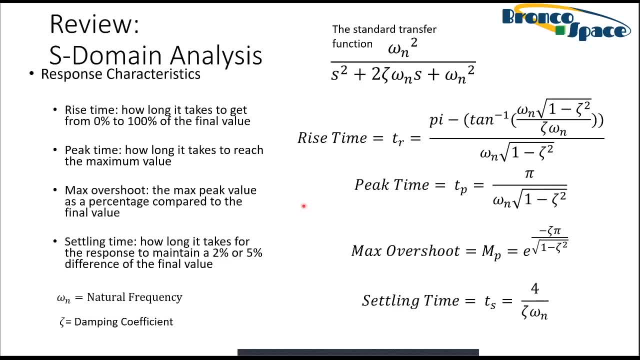 the response of your system based on an input. So you have to remember: right, a control system takes a human input. right, you tell the system to do something like it: fix a thermostat. right, you tell it to go to a temperature. or you know your steering wheel when you turn the steering. 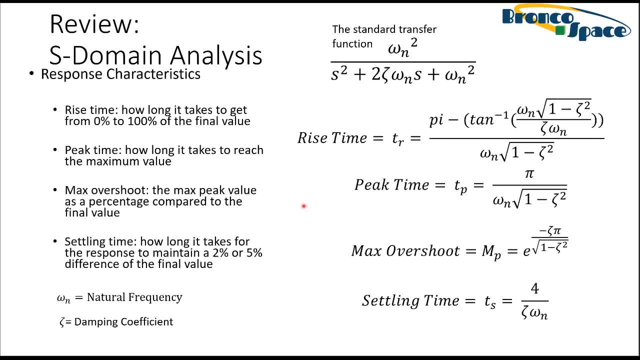 wheel, you're telling the vehicle to turn some certain amount and the control system is the interface between your input and the actual physical you know thing, that action that manifests, And something called a transfer function kind of goes in between them. The 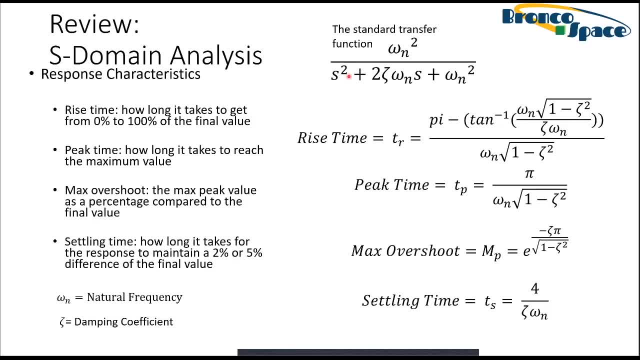 transfer function is like you know, you put in like x at one end and what you get out the other end, x is your input. you know, whatever you get at the output is the output and the transfer function. with this fancy-pants, math can roughly idealize right like how the system is going to respond. 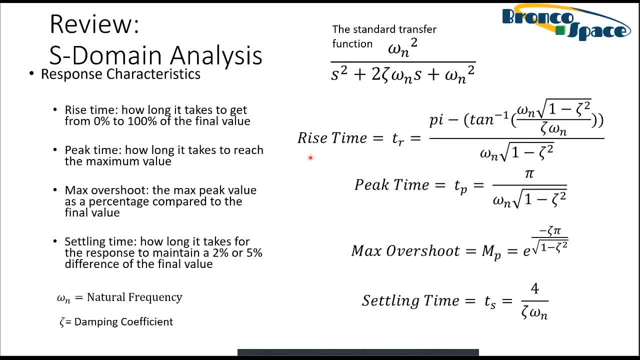 in terms of like rise time, like how long does it take to get to the value you want it to get? like a peak time, right. like how long to get to a maximum value, because sometimes, right like you can have things like overshoot, undershoot, right, how long does it take to settle? 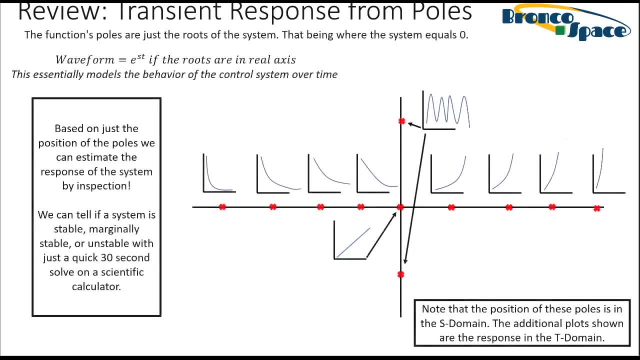 yeah, We'll get into this a little more. not really actually. One of the things that's kind of important to understand is transient response. Now in aerospace, we usually actually use like a continuous time S domain response. Basically, what that is is the system becomes idealized. 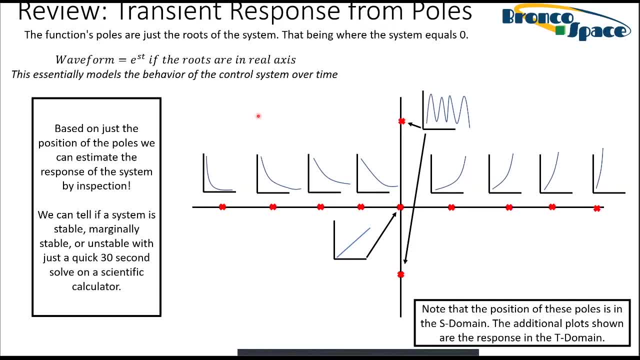 as a continuous function, right like a smooth curve, basically right, where all the all the points are connected to infinity. Real-world systems behave in a continuous manner, but the computers that actually control real-world systems are, unfortunately, discrete right. 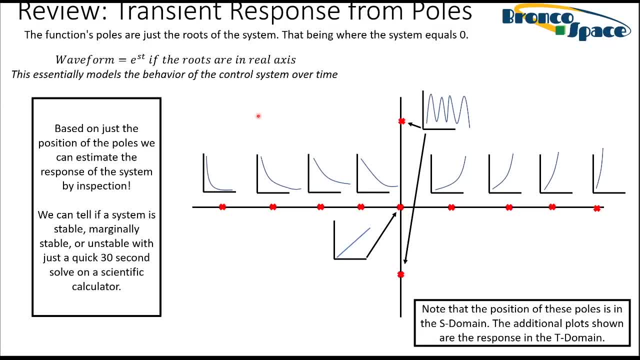 it's all ones and zeros in there, right, and you can have really high-resolution systems that behave essentially continuous, but they really aren't continuous. so when you get really into it, you have to actually discrete time right, and you have to actually get really into it. 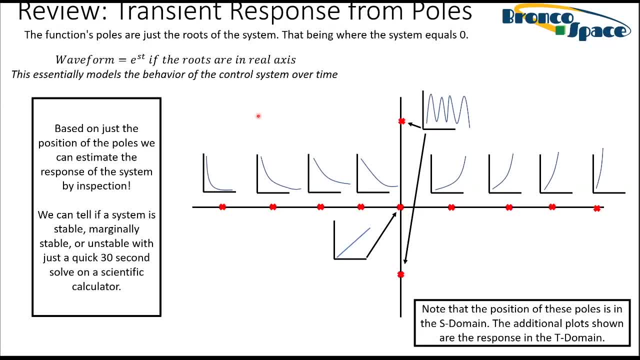 and you have to actually synthesize right all of your sort of equations so that they become little steps rather than just a continuous curve. but no, we're not going to worry about that too much for the sake of this. like introductory workshop, Something important to understand. 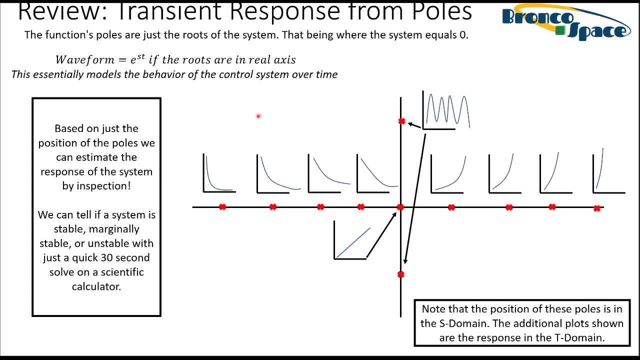 though, is that when you talk about control systems, there are sort of three types where you have like stable systems, and what a stable system is, you can see on this. this is a lot don't worry about, like a position of the poles right now, but stable systems are. 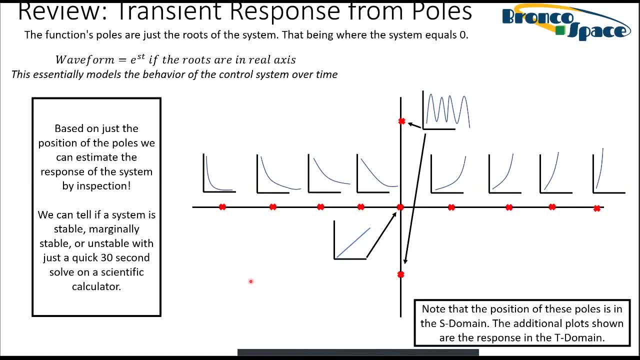 systems where, if you take your hands off of them and just let them do their thing with no intervention, they will eventually stop right, like they are just going to reach a value and they are going to stay at that value. that's a stable system. Then there are marginally stable. 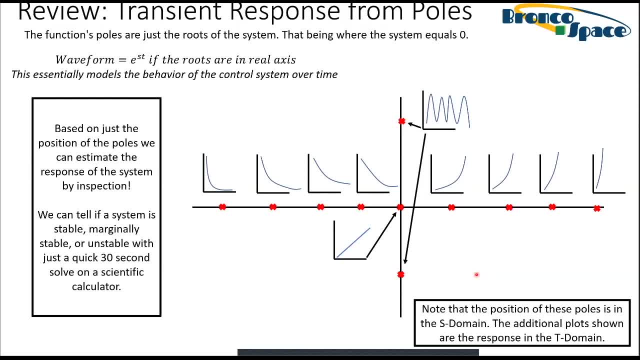 systems. Marginally stable systems are systems that oscillate, so a marginally stable system will forever kind of like just bounce like in between a set of values rather than settling on a single value, and then you have totally unstable systems right which 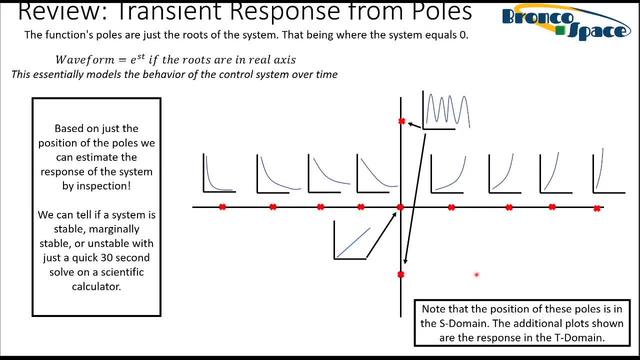 are systems that you get it going and then it just keeps going forever, like it never stops itself from, you know, going in a certain direction. In sort of a rule of thumb is that the more stable a system is, the slower it is to respond to an input, and we usually call that damping. 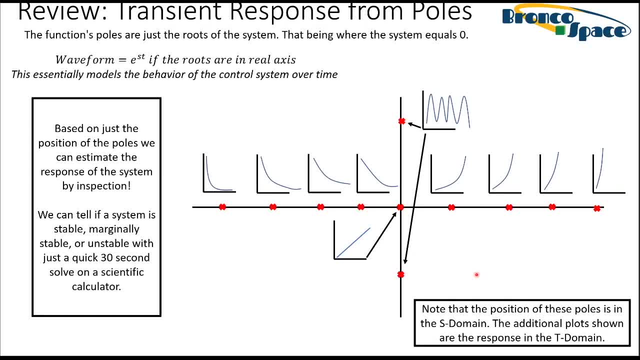 right like a very damped system is a system that is slow to respond to input. but you know that because it's very damped that it won't just go nuts on you and, depending on the requirements of your system, you might want that, you might not want that. 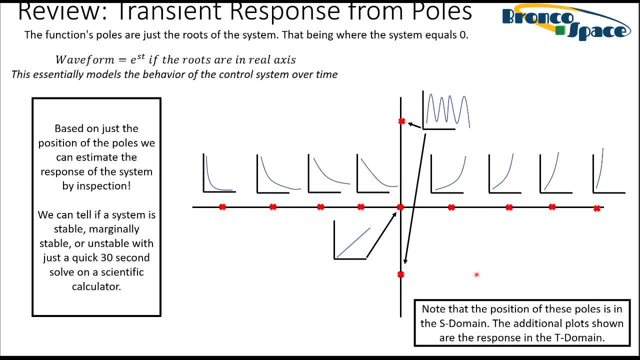 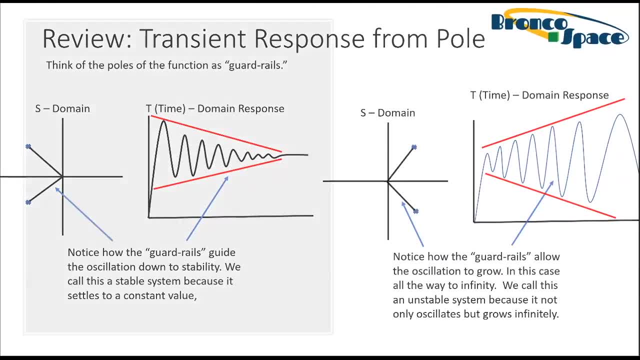 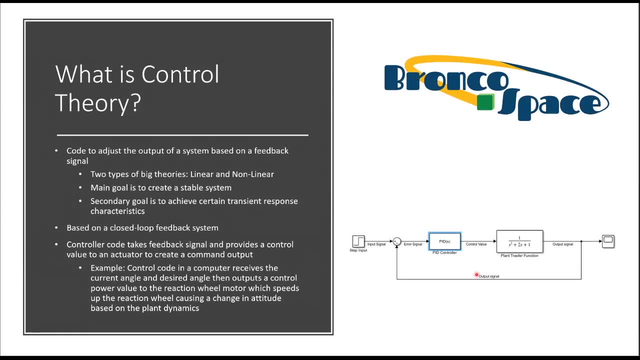 It really just depends on what you're trying to accomplish and how much you trust your control algorithm to sort of figure it out at the end of the day. I'm actually going to skip this, Okay. so control theory right is how we go about actually designing the system. 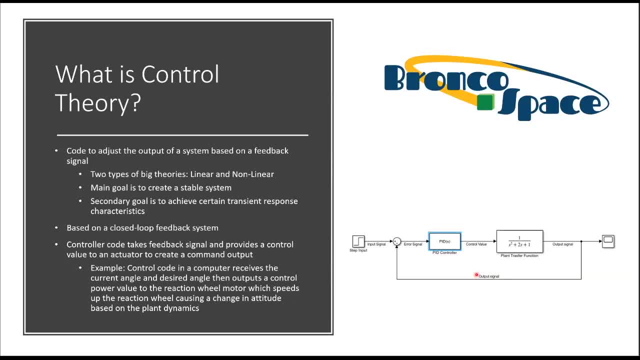 that turns your input into the desired output. And, for the The sake of what we're doing, pretty much everything we do is going to be a closed loop control system. What that means is that you have your input right, your desired value- that goes into the system. you have some sort of controller right that translates your input and tweaks it right so that when it's applied to the plant- which is your physical system- right, 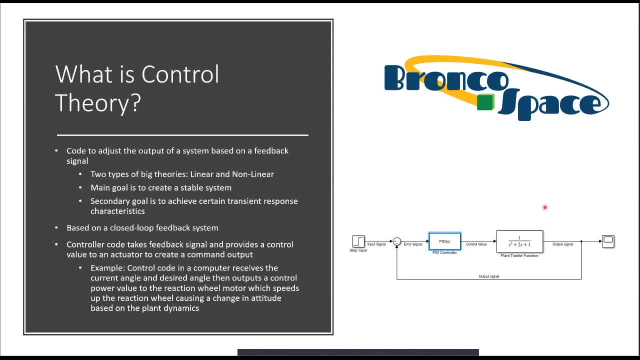 the plant in this case might be like the satellite or the robot arm right or the steering wheel, the car right that has all those physical properties about it produces the desired output. And then the feedback part is that, rather than just going straight through right from input straight to output, there's also a feedback where we take the output as it's happening and stick it back in the system right. 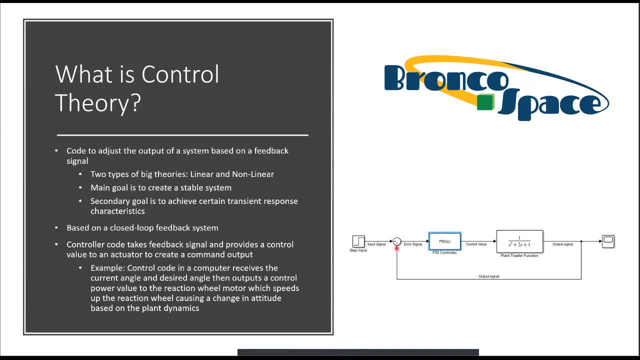 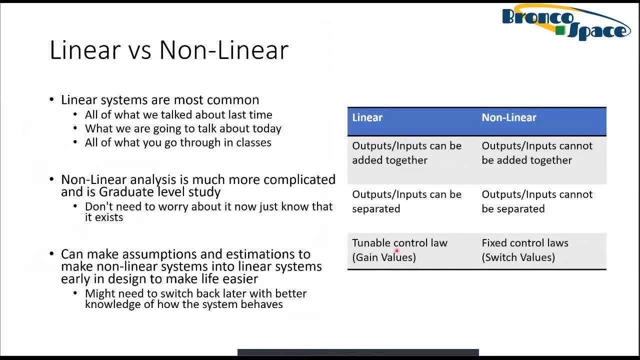 to adjust the response as the system is ongoing. There are also linear and nonlinear systems. We're not really going to get into nonlinear systems at all because they are very complicated and totally beyond the scope of an undergraduate program, And so we're going to just focus on like. 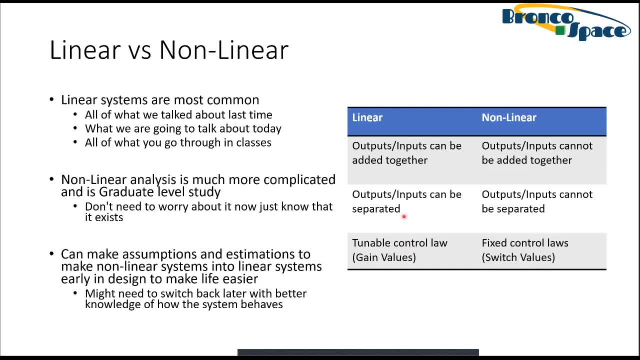 the linear systems for now, And you can generally idealize a satellite system as a linear system and pretty much get away with it, aside from like really precise you know requirement when you have really precise pointing requirements. Sort of a summary here. right is that a linear system is one where the outputs and inputs can be added together and they can be separated. 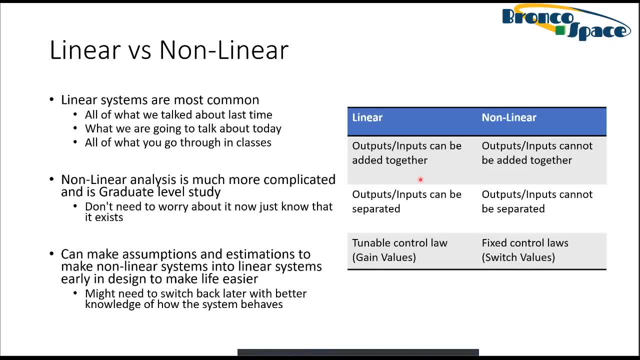 Whereas a nonlinear system is one where the outputs and inputs can be added together and they can be separated, Whereas a nonlinear system is one where the outputs and inputs can be added together and they can be separated. What that sort of means is like. 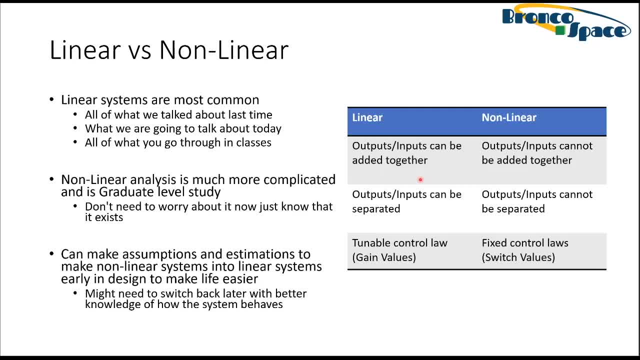 the outputs and inputs being inseparable, are when two physical characteristics of a system are coupled to each other. If I remember correctly, in spacecraft you can sometimes get this thing known as pitch roll. Is it pitch roll or pitch yaw? It's one of. I think pitch and roll are actually coupled. 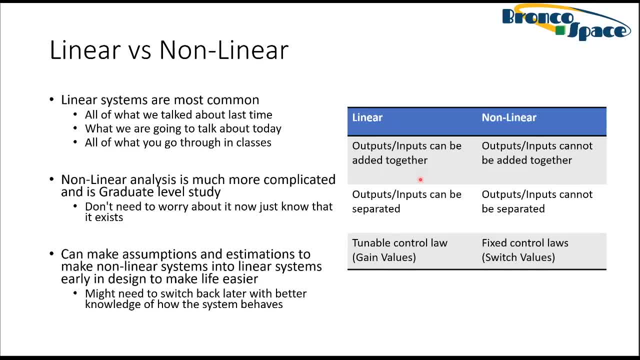 if you have an unsymmetrical spacecraft where affecting you cannot affect one of those of those properties without it also affecting the other. Yeah, Oh, Flynn, were you gonna interrupt me, or Nah, Okay, we're good. Am I going too fast? 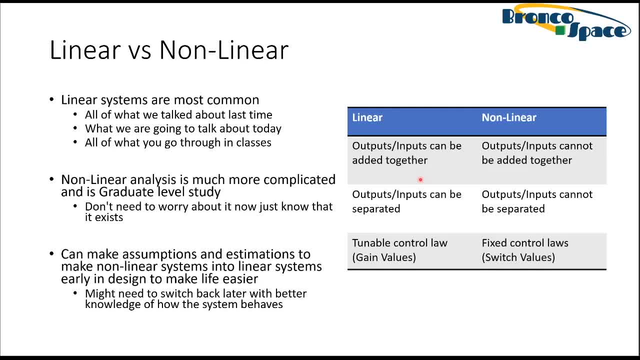 Am I going too fast? I feel like I'm tearing through this, but Yes, no, maybe. actually, I think I can put the list of people over here. So if you guys want me to go slower or go faster, you can just hit the button. 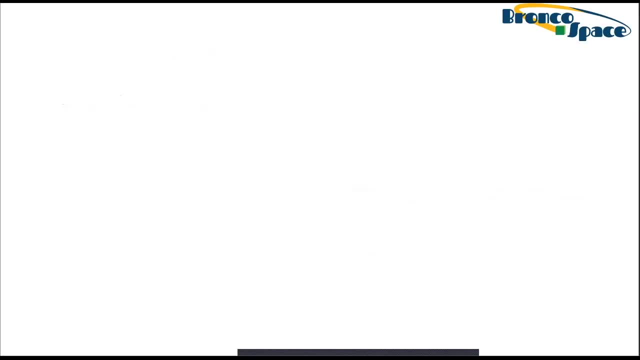 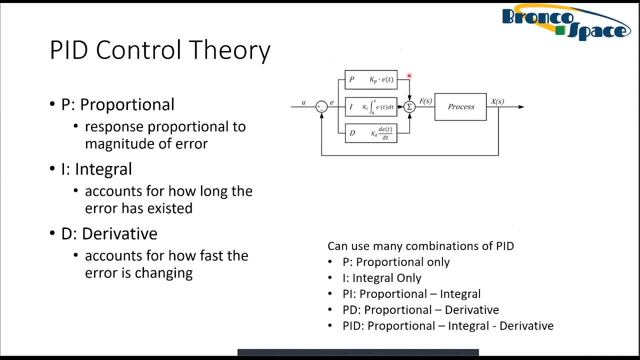 Okay, okay, I'm getting a go faster, So I'm just gonna go faster. There's a closer feedback system. We already talked about that. Now most spacecraft are going to just use normal PID control theory for the actual controller. You might also introduce things like common filters. 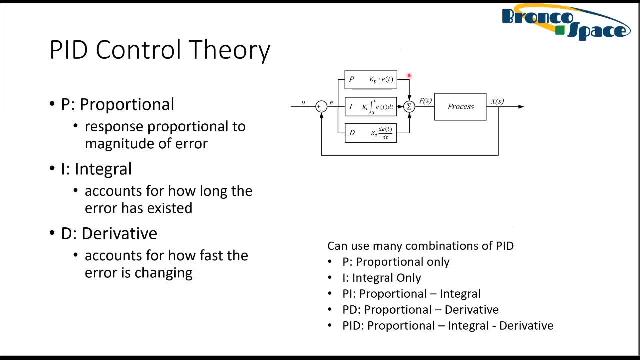 on the discrimination side, but in terms of control for the applications that a CubeSat is gonna find itself in, PID does a pretty good job And in fact oftentimes you can get away with just a PD and forget the I entirely. As quick review for people who have never seen: 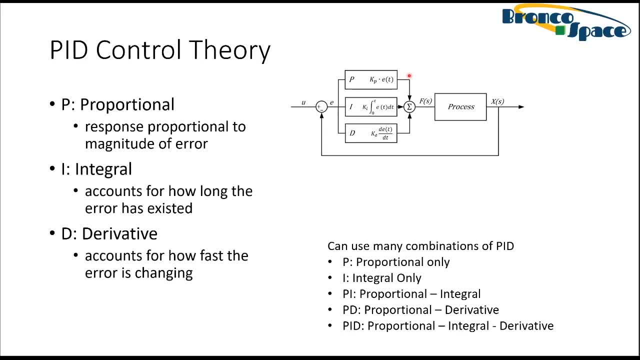 a PID controller before. PID stands for proportional, integral and derivative, And quick summaries are here, right. So the proportional controller just increases or decreases the magnitude of the signal that goes through the system. Think of this as the big multiplication sign. It's bigger or it gets smaller. 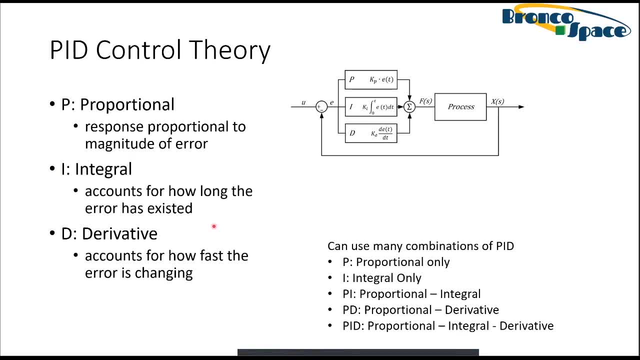 Depends on how the system is set up: Integral accounts for how long an error has existed. So what that ends up doing to the system is if you have like a very small integral accounts for how long an error has existed. So what that ends up doing to the system is if you have like a very small 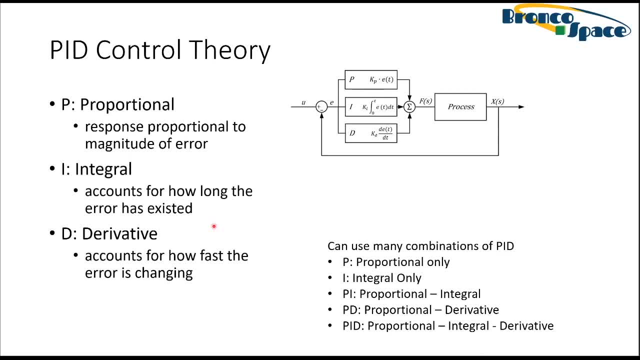 error. like you're just barely right, Like off of the value that you want And it's kind of just there. Like you, your system settles at a value that is not actually the value you want: The integral gain right. 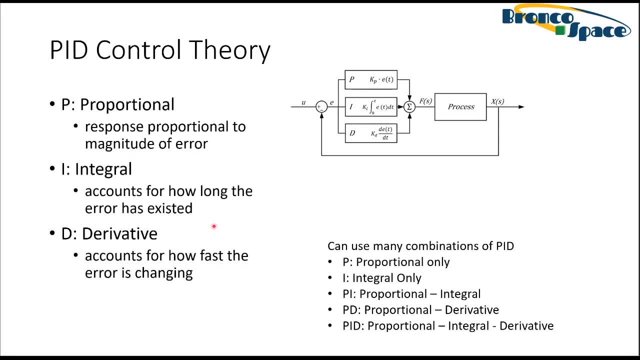 If you turn up the integral, it can get the system to the value you want. The problem is that integral can also introduce oscillation. Derivative, on the other hand, accounts for how fast the error changes. So derivative can smooth out the system. 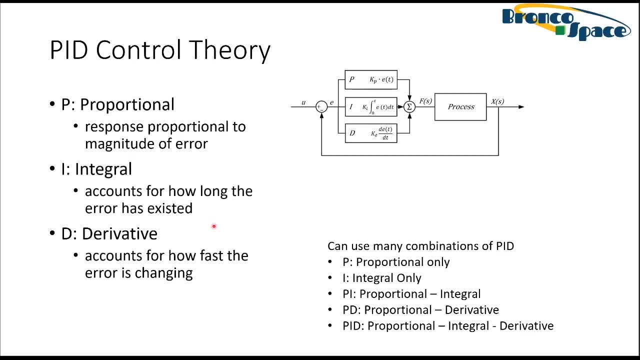 So derivative can smooth out the system If it is oscillating. The issue, though, is that derivative can also just slow down the system in general, because it introduces damping. So it's sort of a balance between all these three values to get the value you actually want. 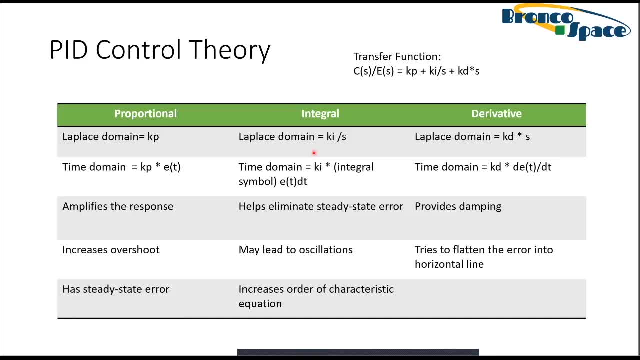 Here's some other stuff where kind of what I was just saying right Like proportional amplifies the response, increases, overshoot, introduces a steady state error, though Integral can eliminate that steady state error, right, Like not being at the actual value you want. 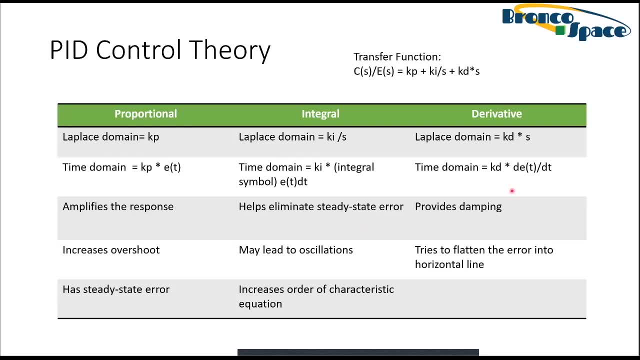 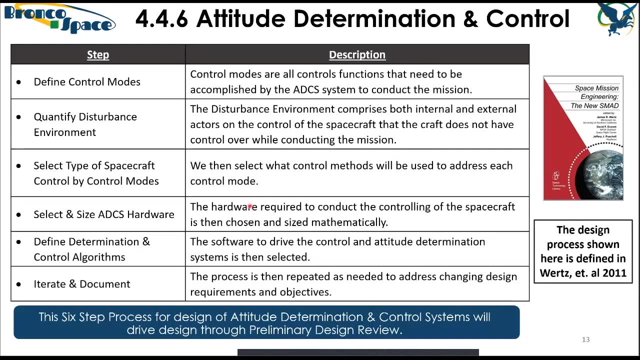 The problem is that integral causes oscillation. Derivative right Provides damping but it slows the system down, So it's a balancing act between all of these values. Okay, so here we get into the actual process of designing a control system. 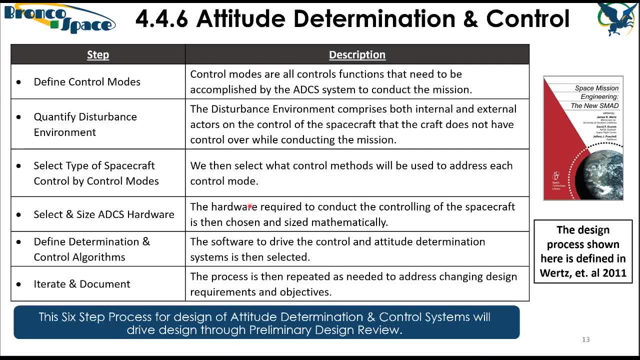 For a spacecraft. Before I go here, though, that was my rapid fire. like 15 minutes, an entire semester of control theory just kind of shoved at you. Is everyone okay with what I just all went over? Like there are questions. 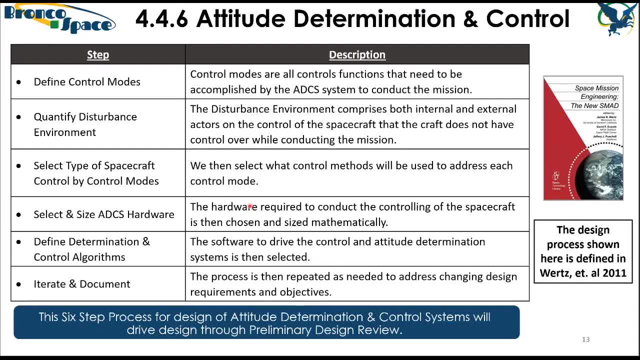 I can visit some questions right now. or if anyone didn't understand anything, All right, I have a thumbs up and a green check, So I'm just gonna say we're good And keep going with it. So I'm gonna take a quick drink of water. actually, 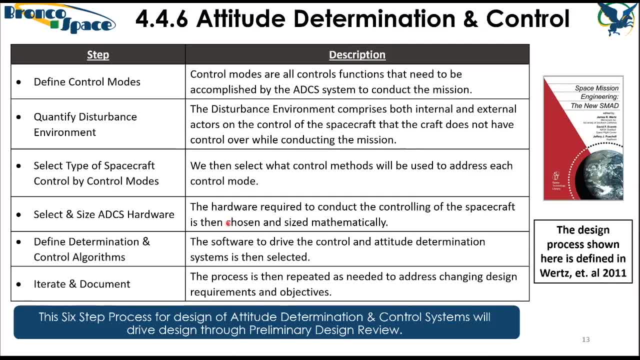 Okay, so you understand basic control systems now, or at least you're too confused to ask any questions, So we're just gonna go ahead and jump right in the even deeper end of the deep end and talk about how we actually put a control system. 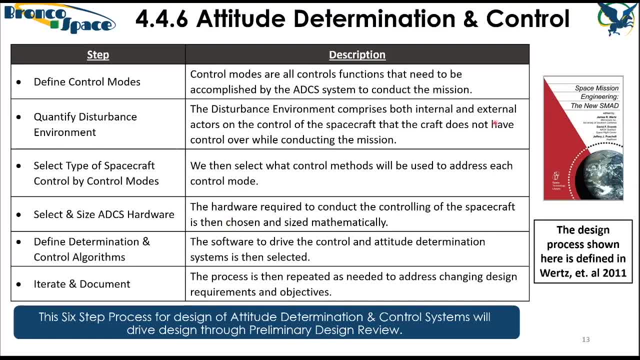 on a spacecraft now. For those of you who are not familiar with the SMAD, it is the Space Mission Analysis and Design Textbook. The latest version works at all 2011.. I don't actually have my copy in my room right now. 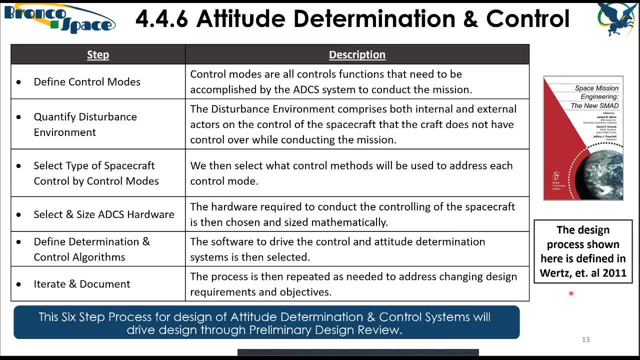 to hold up for you to see, but it's like 1100 pages worth of what can be considered the Space Mission Engineer's Bible And the sort of process for designing an attitude-driven control system. it's actually described pretty well in the textbook. 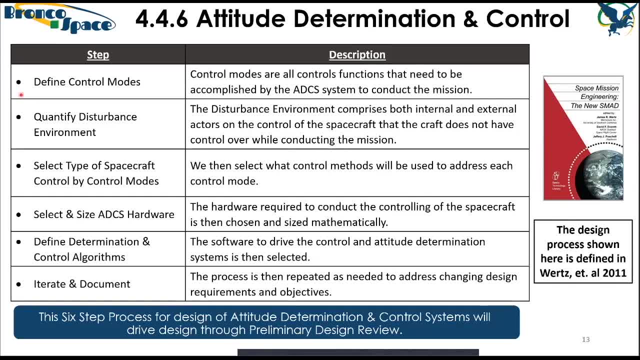 And here it is. there are six steps, and you're gonna sort of iterate through these steps as you build out the system. So the very first thing you need to do, and the most important thing, is define your control modes. Now, what does that mean? 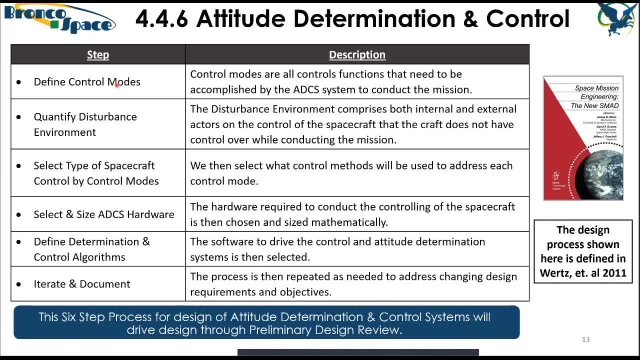 This comes from an understanding of what your mission actually is. Just as an example, like: say, you have a mission that is earth observing, So satellite has a camera. right Now you have to ask: okay, what is the camera going to take pictures of? 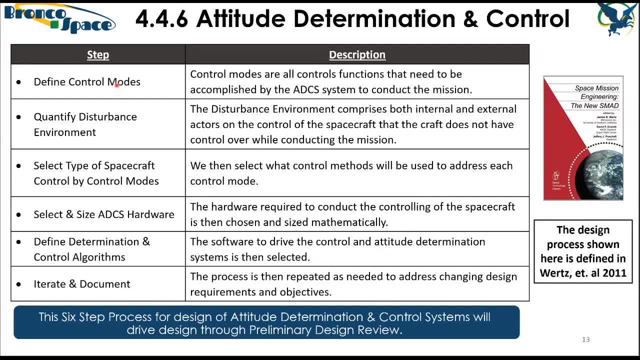 We wanna take pictures of the earth, right, Let's just say we don't really care too much about, like, exactly what on the earth we're taking pictures of. So the control modes are pretty simple. right, You have a control mode where the system is going to try. 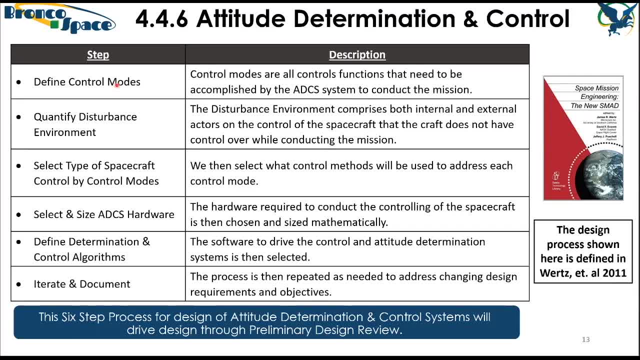 to point the camera at the earth. That's one of your control modes. Now you also have to think about like okay is like: do I need the camera to be tracking an object on the earth, or does it just need to be pointed in the general vicinity? 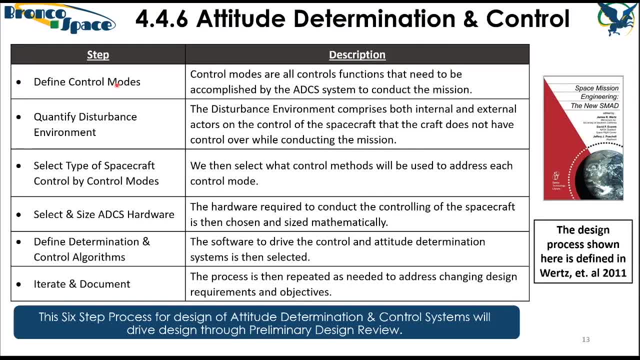 Right and that kind of hones in like: what does the controller actually need to do? Another control mode that's really popular in spacecraft is a sun pointing mode, because it's very uncommon for CubeSats to have articulating solar panels. 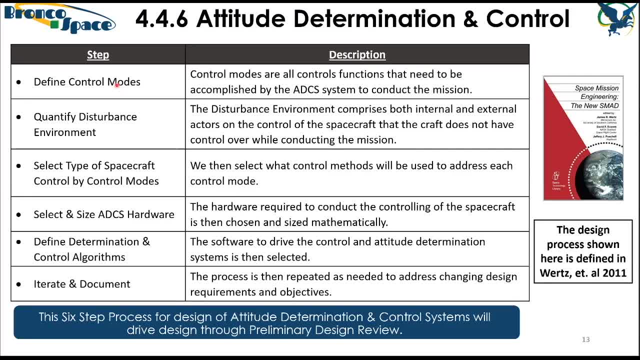 moving parts and reliability don't really go with the whole low cost paradigm. If, like let's say, one face of your satellite has a lot of surface area with solar cells on it, you might want a control mode where the spacecraft will make sure that face with all the solar cells. 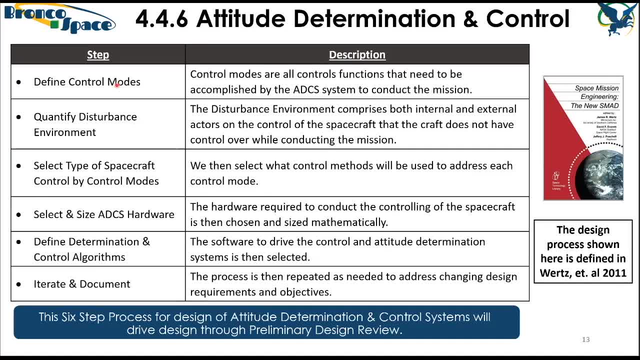 is pointed perpendicular to the sun to get maximum power generation. Or you might have a mode where you have a patch antenna, which is a directional antenna And that needs to be pointed at the earth in order to actually send down all your data. 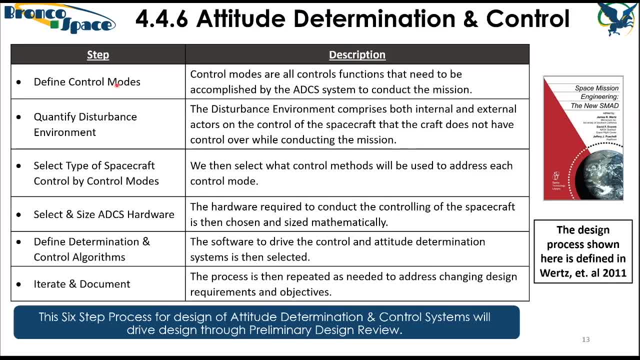 So these are the control modes. You need to define what the control modes are first, because understanding what the control system needs to do is how you actually get down to selecting what is appropriate to be on your control system, Which is where you need to move your camera. 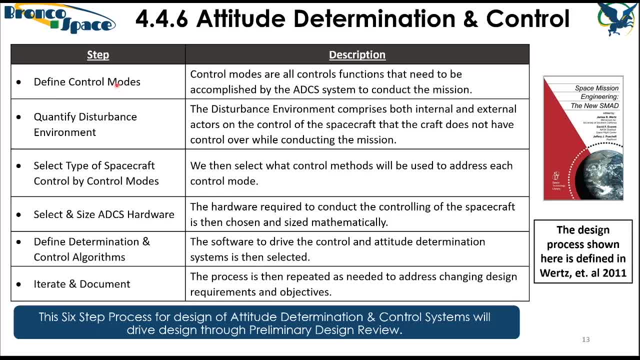 right, Oh, Restart ницу. See, OK. The next thing is you need to quantify the disturbance environment. This actually is not that important for CubeSats, because for a craft as small as a CubeSat it is pretty inconsequential, assuming that you have a control system at all. 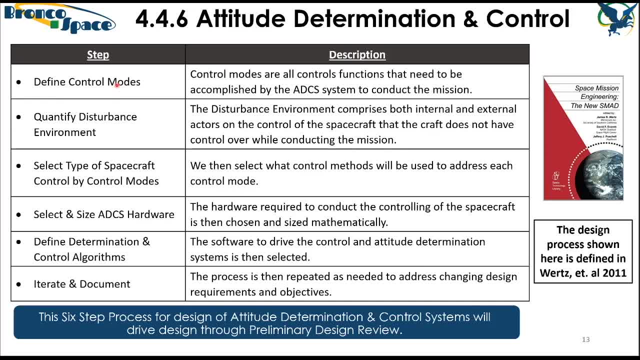 Pretty much any control system will be able to overcome the disturbance environment. This is really only a big issue with like really big spacecraft. Let's say you're like the Hubble Space Telescope with like huge solar arrays. Atmospheric drag can actually be like a significant problem for you, right? because those solar arrays act as massive- well, massive in quotation marks- drag sails. 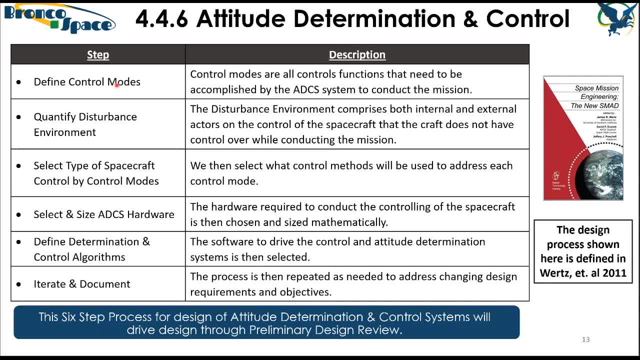 For CubeSats, though they're so small, you generally can just get away with it. You don't have to worry about the disturbance environment so much. One thing, though, that you do need to remember is that the magnetic disturbance environment is oftentimes the worst one for CubeSats. 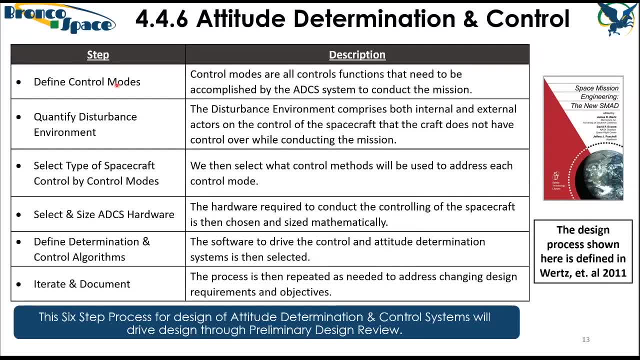 Like. especially if you have, like, anything that's magnetized or magnetorquers on your spacecraft, The magnetic disturbances can actually there are known cases where magnetic disturbances have thrown CubeSats sort of really out of whack. Right, Right. 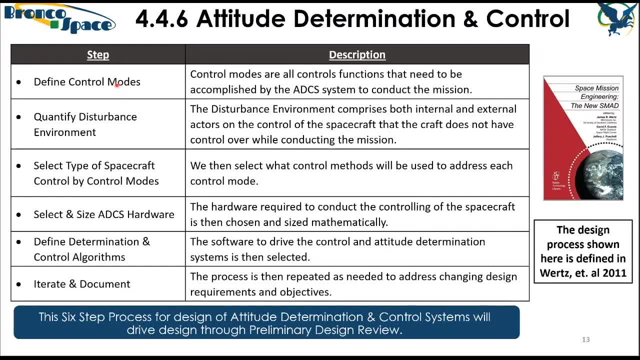 One famous example that I always bring up is the Move2 spacecraft from the University of Munich. They had a wiring issue that they did not know about. They didn't know it was going to be an issue before they launched. Essentially, what it was is like the wire that came from their solar panels into the spacecraft created a wiring loop. 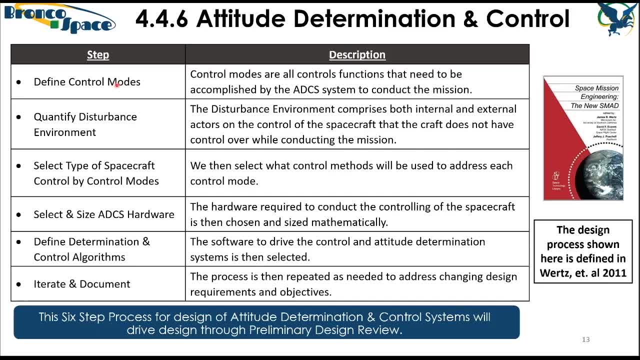 Well, like created a loop right, Like the electricity flowed in a loop around this wiring And that ended up creating a very weak electromagnet on the spacecraft, Like when it interacted with the magnetic field. it caused the spacecraft to go out of control and spin up to a hilarious speed of 500 degrees per second before they were able to get it back under control due to some cunning control engineering. 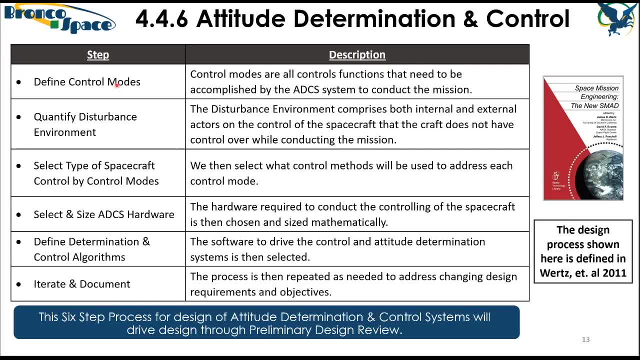 But stuff like that you have to watch out for. Next, you select the actual actuators, right That go. yeah. you select the type of control that you use, depending on the control modes. So in traditional spacecraft engineering there are things like spin stabilization, right. 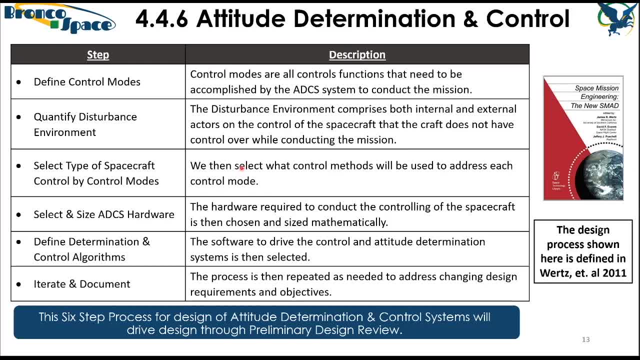 And other you know weird methods- yo-yo, d-spin- You don't really have to worry about those because they're pretty far out there for CubeSats. But types of control that you'll probably hear a lot are things like: 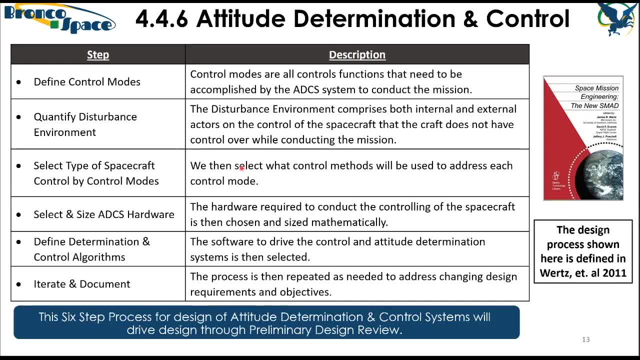 Like you know, de-tumble right When you first come out of the spring-loaded box like your satellite is finally free and in space oftentimes there's a little bit of tumble action going on there Or you know, God forbid, you're one of those poor CubeSats that gets just yeeted off the space station by a cosmonaut, right. 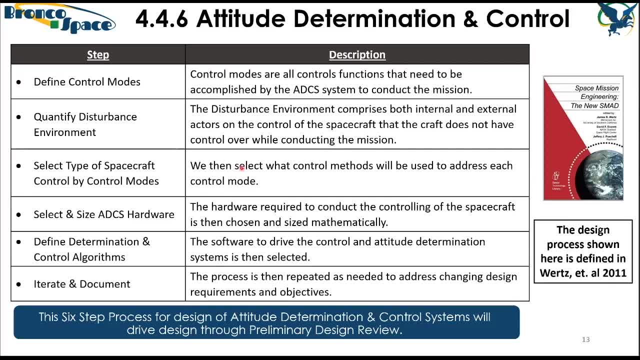 Then there's a lot of tumble that you're going to have to smooth out of the system before you're able to do anything else. So, yeah, So the control methods are- you know words like de-tumble right, Where we try to go from an uncontrolled spin to a stable- just we're vibing, right. 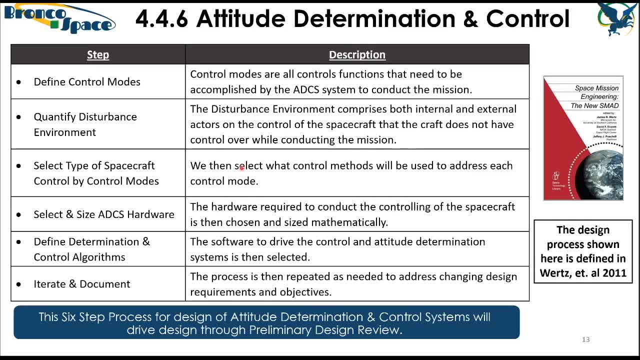 We're just floating. There's no angular movement here. There are things like just normal pointing right, Where we just try to point at a target. There's also tracking right Where, like, there's a point on the ground, for example. 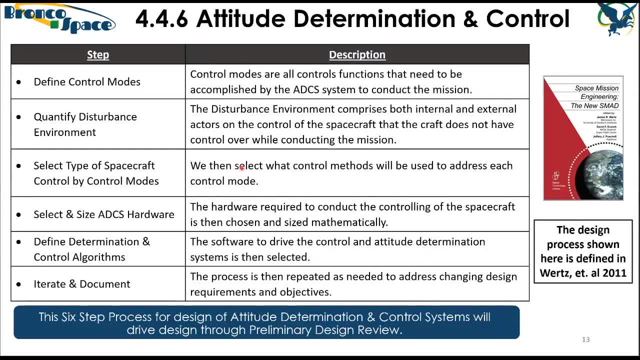 And as we fly over, we try to, you know, follow, follow that point with the target. There's a point with the spacecraft. Once you understand what your spacecraft needs to do, you can actually go to select and size your hardware. 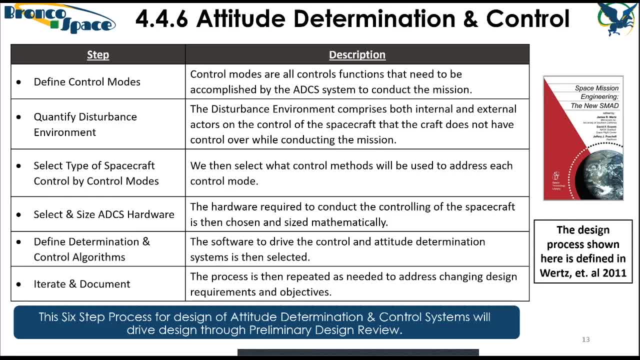 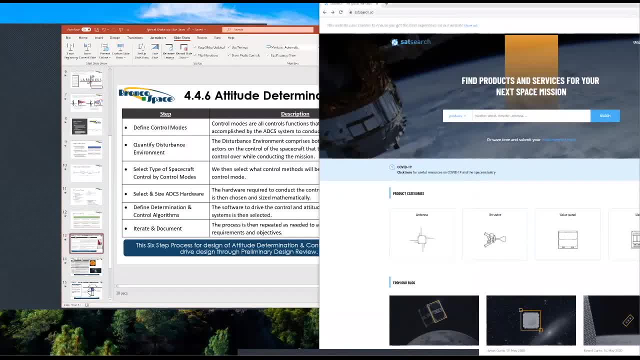 And we're going to do this portion. I'm just going to show you some stuff, kind of live actually. Oops, I didn't mean to do that. I'm just going to kind of show you this live, So not sponsored by SacSearch. 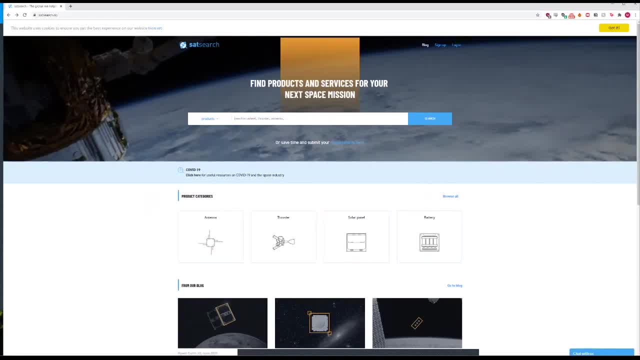 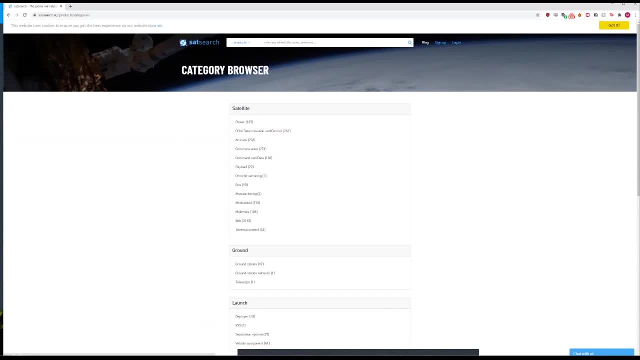 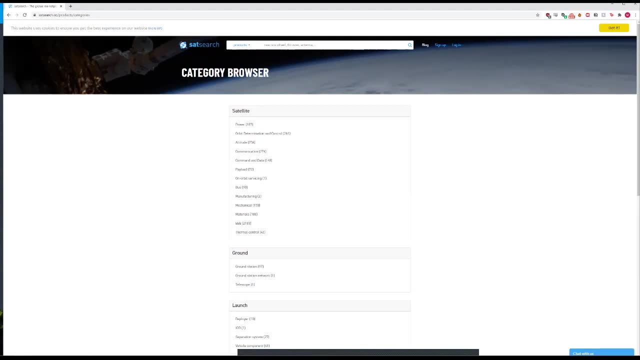 They are. They do represent the Blue Dot Consortium, But they did not pay us any money to use the website. I just think it's the most convenient. They're like I mentioned earlier. there are a couple different types of actuators that can be used in a satellite control system. 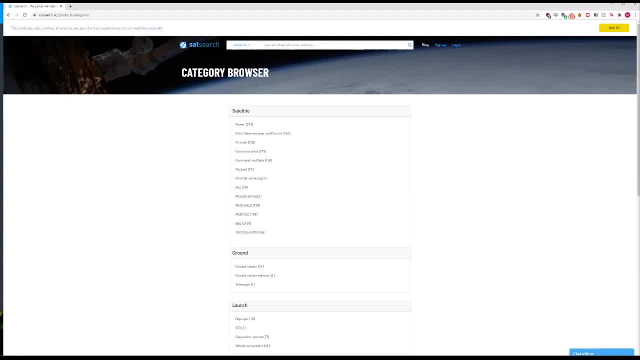 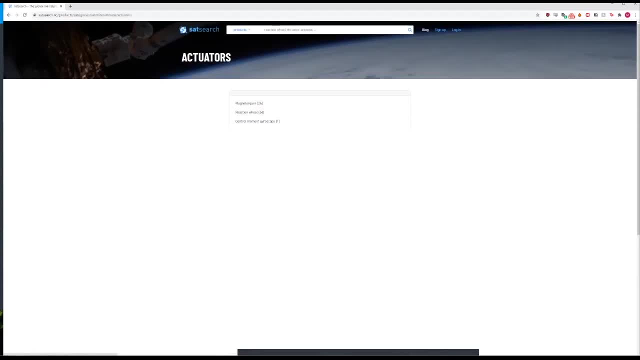 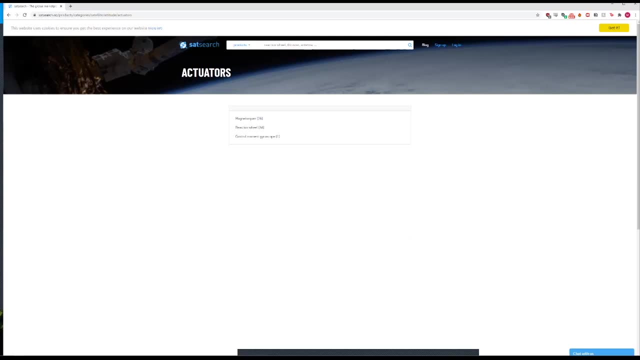 Now an actuator- remember is the device right that takes the input and makes the physical change in the system. So we go in here to attitude. You can see actuators. Here are There's three options here. but really like control moment, gyroscopes are kind of the same thing as reaction wheels. 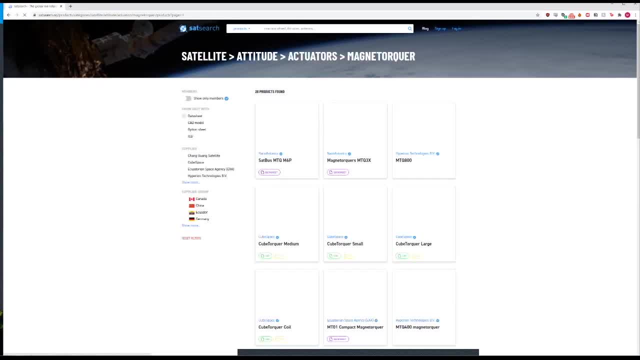 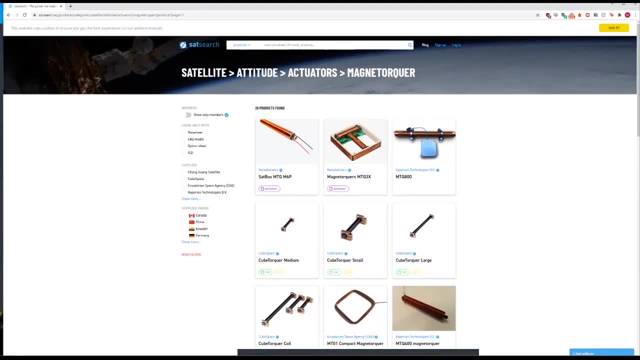 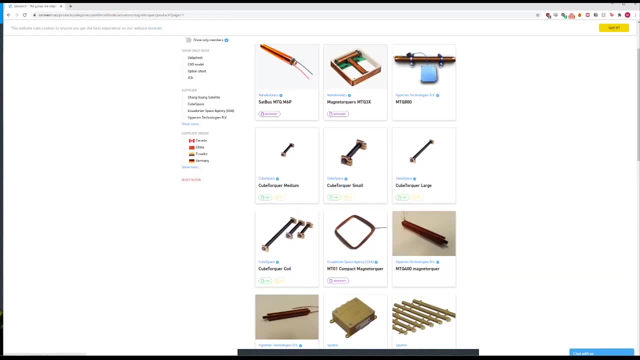 The most common is magnetorquers And I think the statistic is like 80% of CubeSats have magnetorquers. now, What these magnetorquers do is they essentially turn your CubeSat into a compass. Magnetorquers are characteristically just either a coil like this right 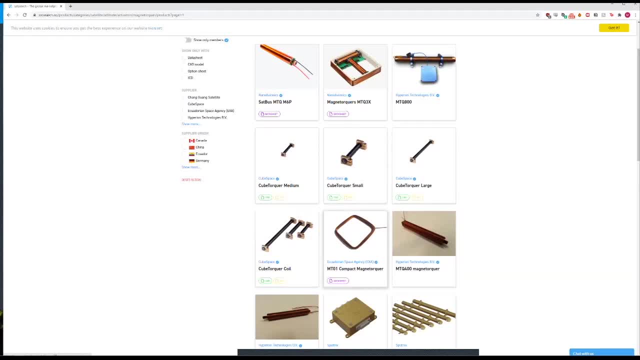 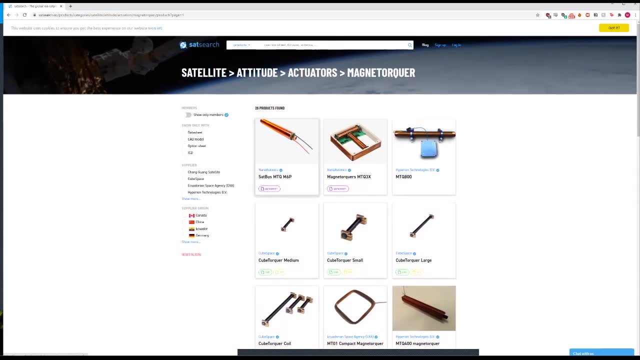 Just a literal coil, A literal coil of wire. Or they are a rod, sometimes called torque rods that are also a coil of wire, but they might have like an iron core in the middle. And what these are? these are electromagnets. 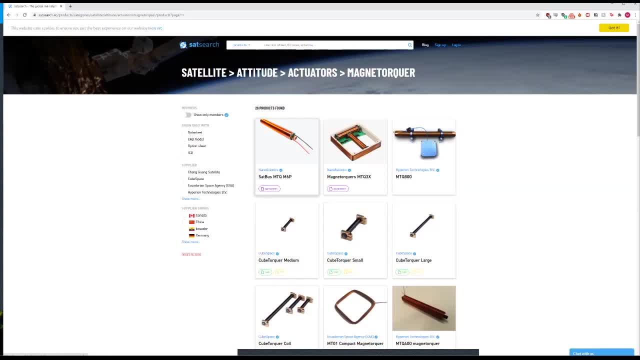 If you remember from your like high school AP physics class, right, you run a current through a loop of wire and it creates a magnetic field And that magnetic field that's created can then interact with Earth's magnetic field And that actually will create a torque on your spacecraft. 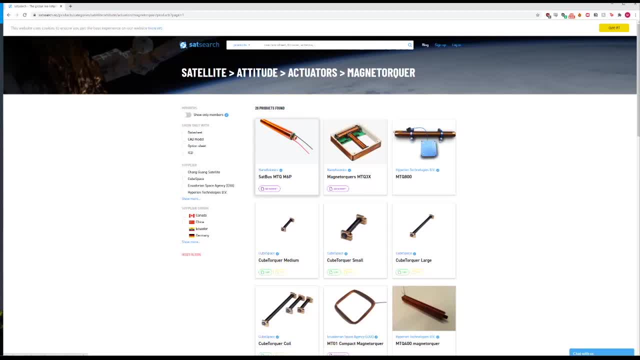 Now it's important to note that this is a torque, not a force right, So magnetorquers cannot physically move your spacecraft. like translationally. There's no forwards or backwards with the magnetorquer, There's only spin, right. 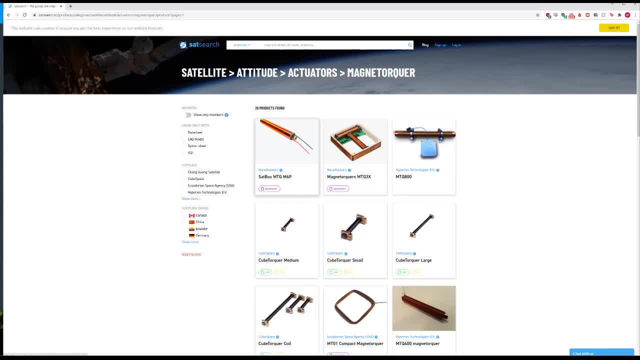 And so it can induce a spin in your spacecraft And that can allow the spacecraft to say, from a spin Right, It can remove the angular momentum and detumble it, Or it can, you know, slowly guide a spacecraft towards a pointing orientation. 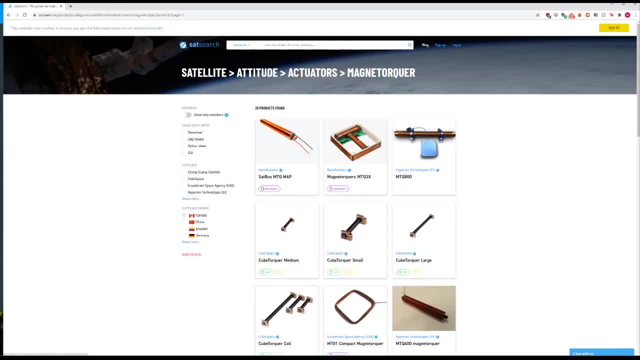 Right, All by interacting with Earth's magnetic field. The pros of magnetorquers: they're relatively simple, Right. It's literally just a coil of wire that you run a current through. So they're pretty foolproof And they're easy to implement. 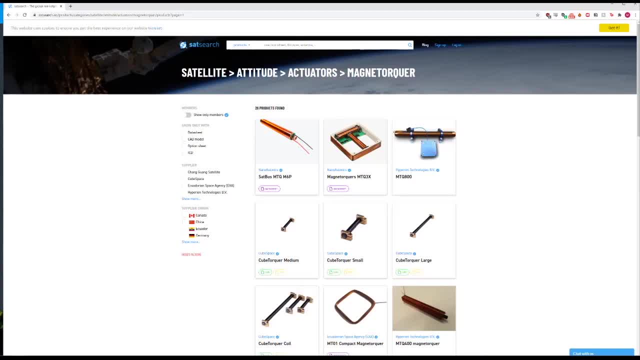 They're also very damped, Which are depending on your Depending on your system could be good, And what that means is that they generate such a small amount of torque that you move pretty slow with magnetorquers, So it's hard to screw it up. 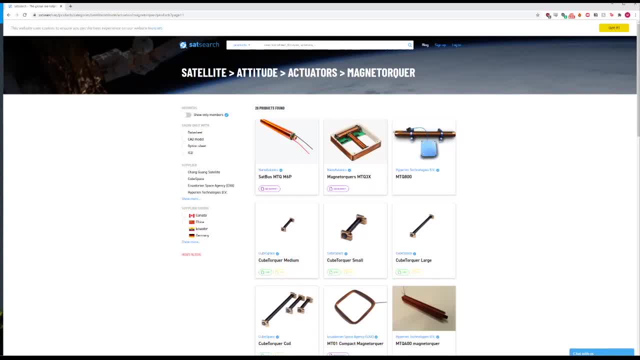 Right Like. there's going to be no situation where you're just flopping out of control with the magnetorquer because the control system has freaked out. In fact, If the System gets stuck Right, Like if the magnet is just always on, 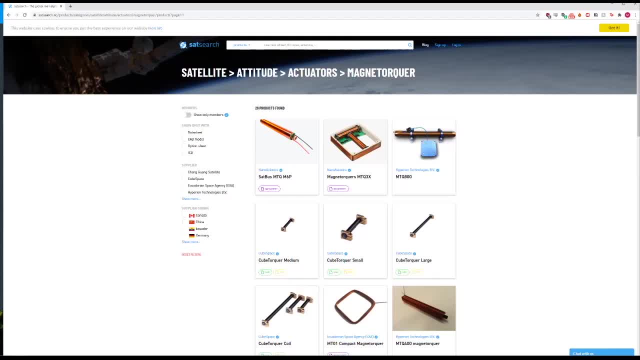 That can actually be good, Because then it just turns into a hysteresis rod. What a hysteresis rod is is just a literal permanent magnet that just makes sure the satellite doesn't spin out of control, Because it's always trying to align itself with the Earth's magnetic field. 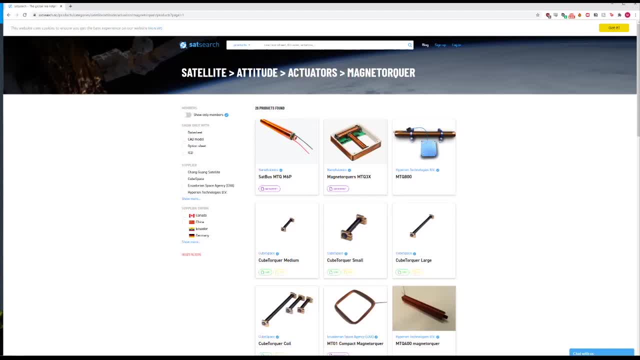 So it eventually reaches a state of stability. Hysteresis rods are kind of like eh Like. don't do them in the CubeSat industry, Because a couple years ago a couple CubeSats got stuck together because of permanent magnets and lost both of the CubeSats. So yeah, But magnetorquers are becoming pretty commonplace. They don't actually have to even be like these independent systems. It's becoming increasingly popular to actually embed them inside, like the solar panel. PCBs, as like just a really thick copper pour in the shape of a spiral. 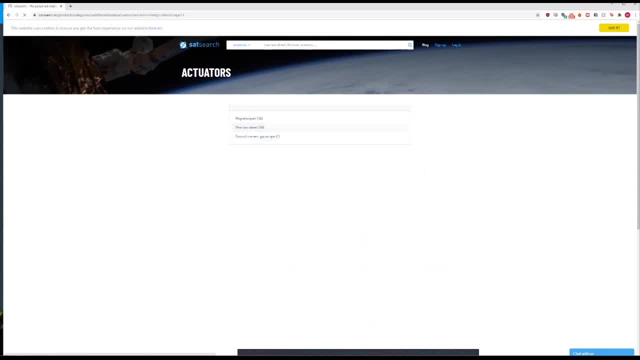 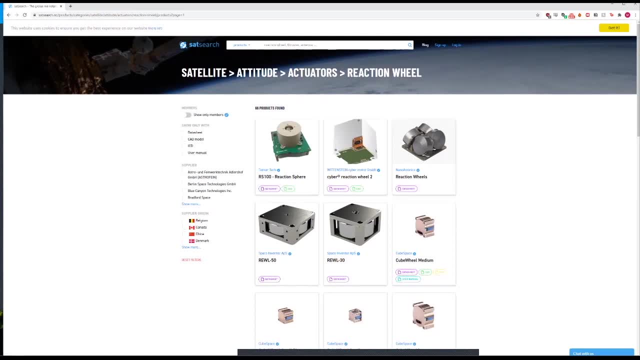 Those are magnetorquers, The other are reaction wheels. Reaction wheels are the more traditional way, to you know, have your spacecraft torque about. If you remember to your physics class back in high school at some point your teacher probably had you had someone in the class sit on a rolly chair, hold a bicycle wheel right in their hands that was spinning right. 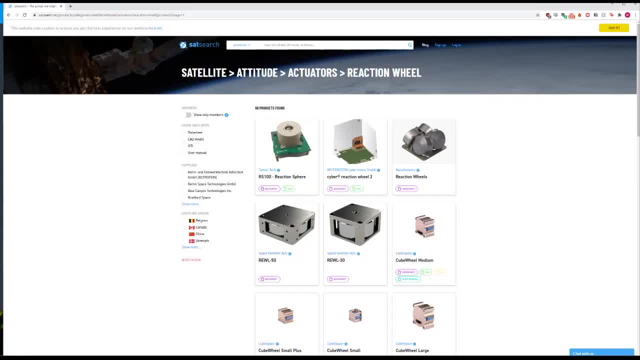 And when you hold it like straight up and down, no spin. When you turn it this way, When you turn it this way, right, Like the magic happens and then the angular momentum starts spinning you in the chair. Same thing, basically, with reaction wheels. 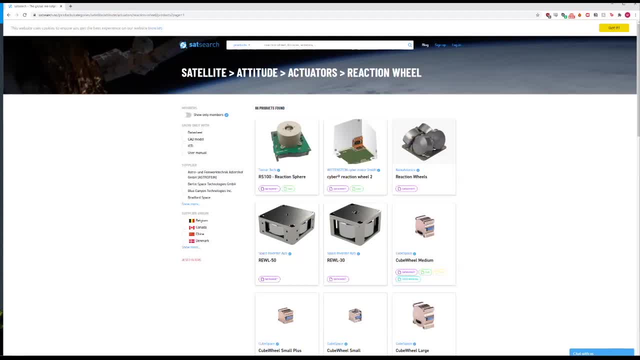 Where they spin in themselves right, And when that spin speeds up or slows down, it transfers the torque from the wheel into the spacecraft right through the whole conservation of momentum thing. Reaction wheels are great because they can move the spacecraft really fast. 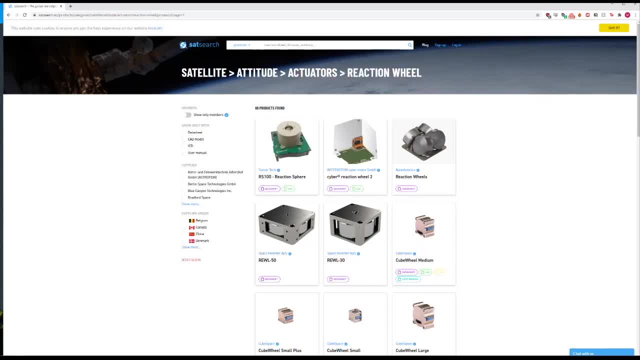 Like they can be pretty snappy And they can also achieve much more accurate pointing with compared to magnetorquers, because they're not dependent on Earth's magnetic field. Earth's magnetic field is actually like, really nonuniform. It has a lot of like lumps and it's inconsistent. 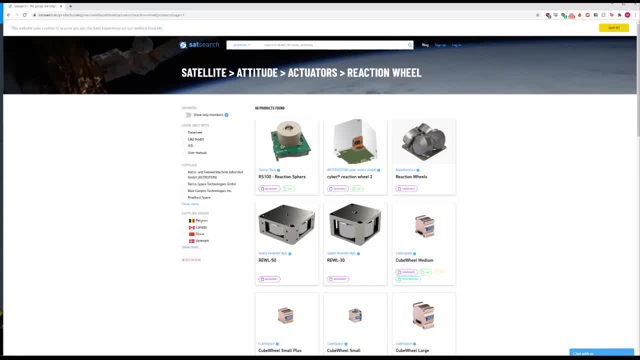 Which can make the performance of magnetorquers vary a lot depending on where you are relative to the Earth. Reaction wheels, they pretty much always work the same. The problem is that they are hilariously expensive and they take a huge amount of your spacecraft in order to actually- you know- fit them in there. 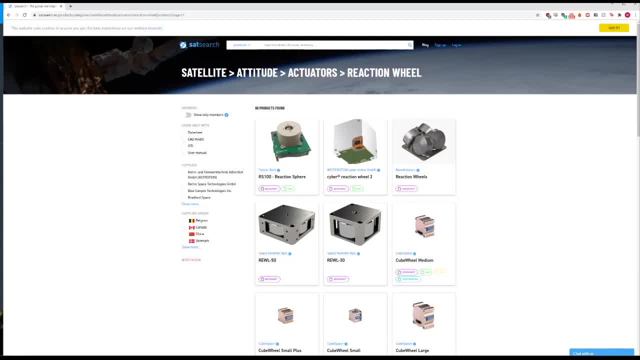 But if you're in a high performance operation where you need accurate pointing, they're really the only true option you have. There's also the control moment, gyro. Oh, I should say that usually reaction wheels come in sets of five Right, Or sets of three. 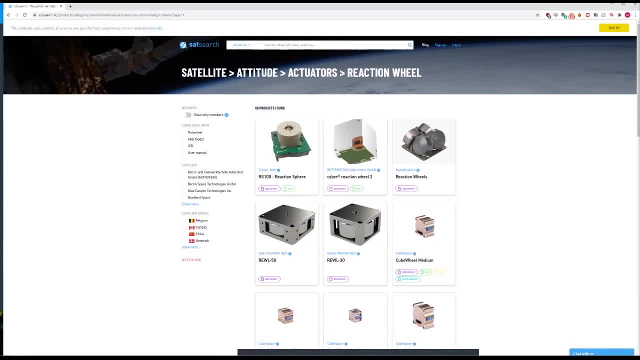 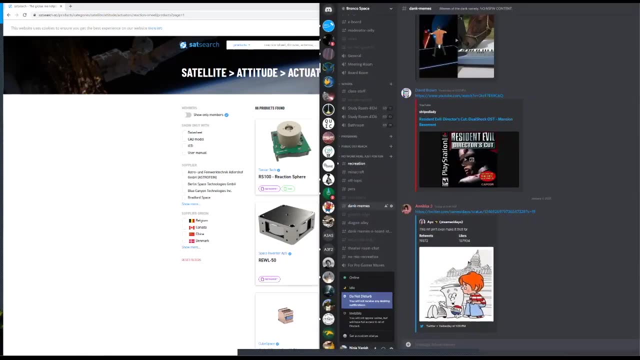 Because you need them to be orthogonal to each other, So one reaction wheel is able to act on each of the three axes: right, X, Y and Z. Yeah, Hold on, I'm going to silence my notifications because this has been pinging like the entire time. 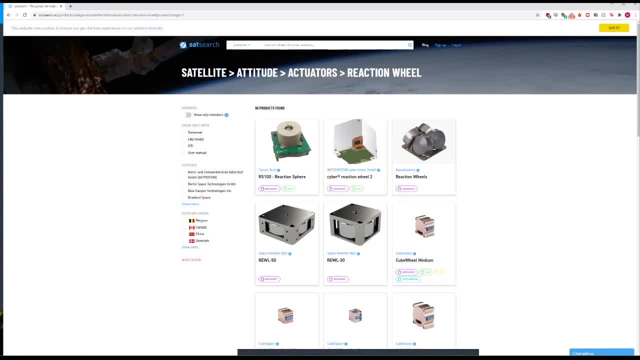 All right, Yeah, Sorry, I was putting a meme. Oh, okay, No problem, Flynn. Yeah, So usually you want three reaction wheels. Sometimes you have systems like this where there are four reaction wheels, not orthogonal to each other, And that's so that if one of the wheels fails right, the other three can still pick up the slack and maintain control of the satellite. 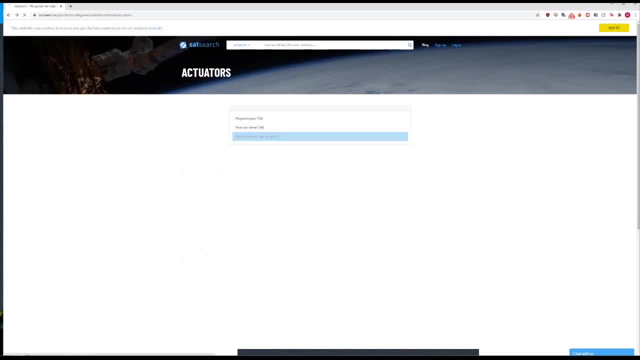 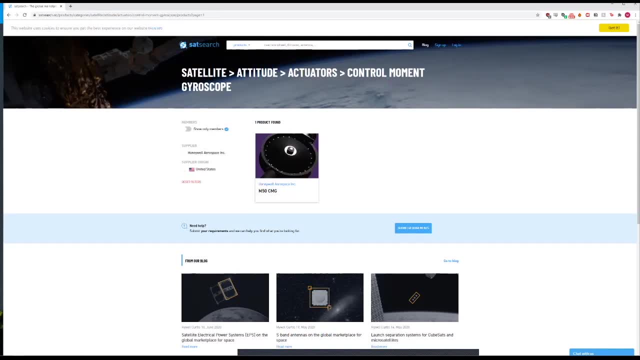 There is also the control moment gyroscope, which is essentially just one reaction wheel in an axis that you care a lot about, And I'll show you an example of what a control moment gyroscope can do a little later. But this is a more sort of unconventional take on how to do the control system. 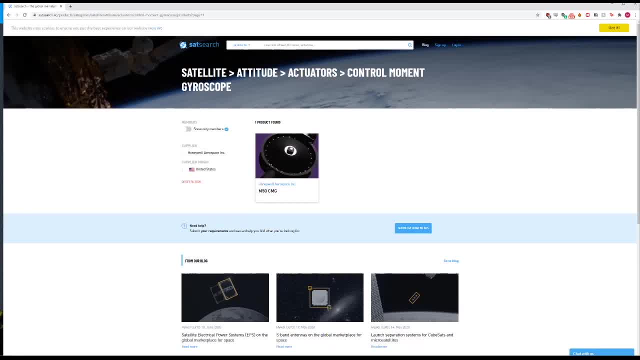 Michael, have you shown the reaction sphere? Oh, like the YouTube thing. No, no, no, It's on SatSearch. Oh, it is. I mean, it's probably on YouTube. Is there a reaction sphere? They have one. 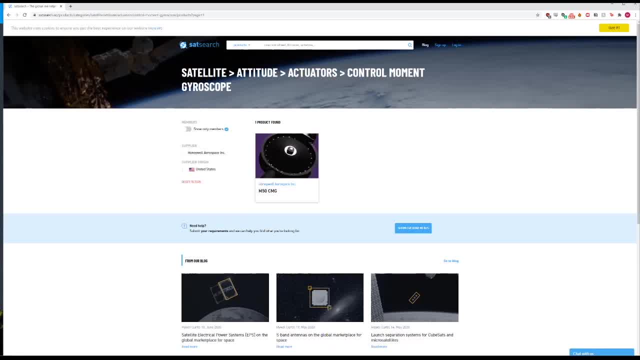 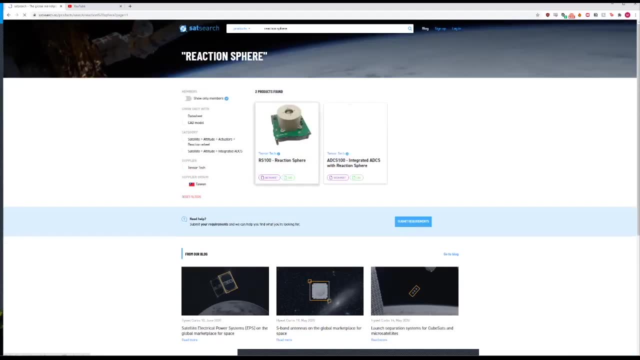 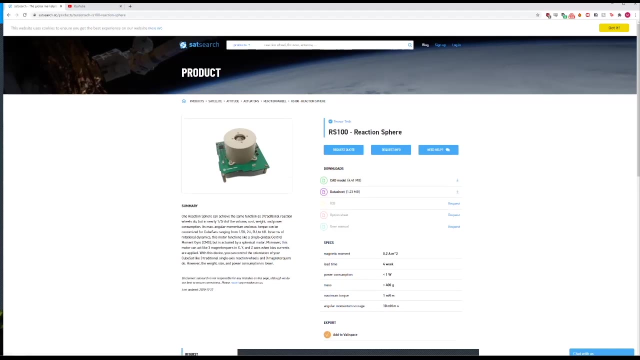 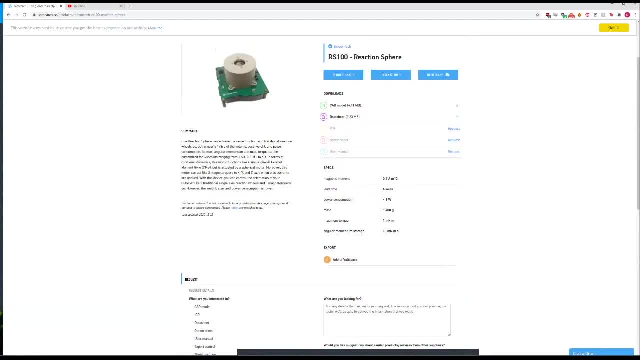 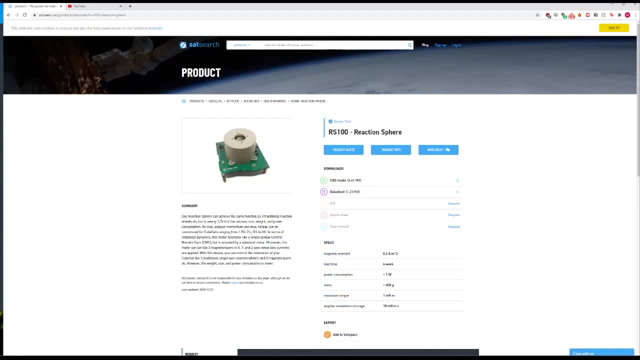 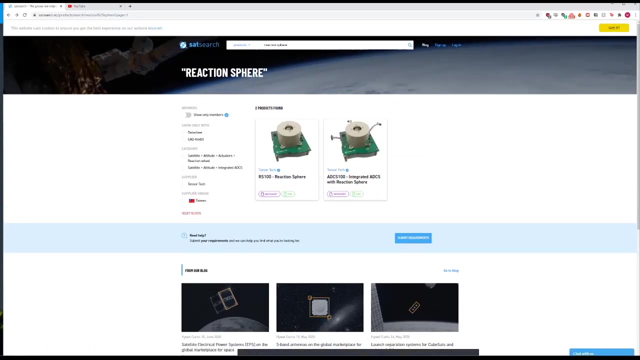 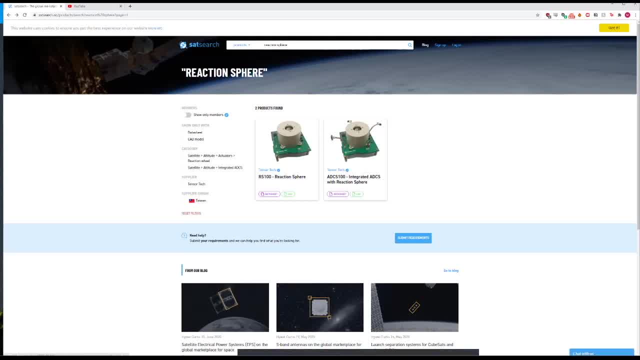 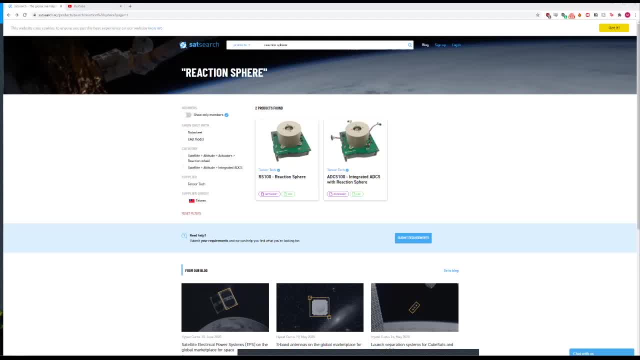 wait, i'm sorry you were breaking up a bit there. my mute button was like going wild. um, sorry, i i just wanted, like what's the what's like? the comparison in speeds? like is so it doesn't take like a magnetor like hours to rotate in the right direction, compared to like a reaction. 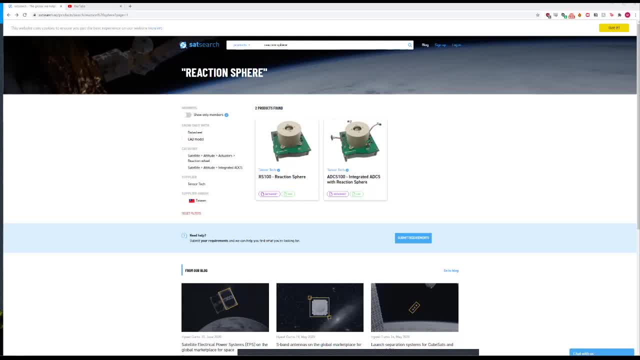 wheel which gets you in seconds, or is it more like minutes? to like minutes? yeah, um. so the unfortunate answer that is the most true is that it depends, but the answer you actually want is probably that, uh, i think top of my head like the back of the napkin calculation. 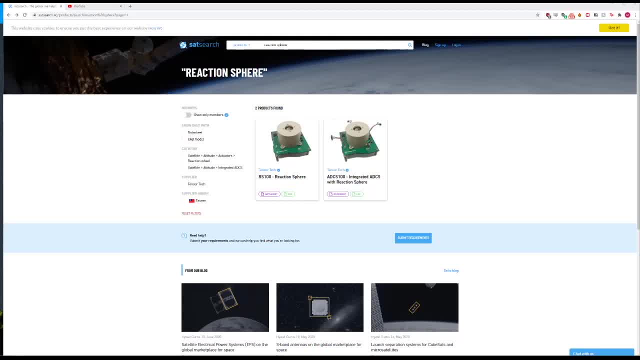 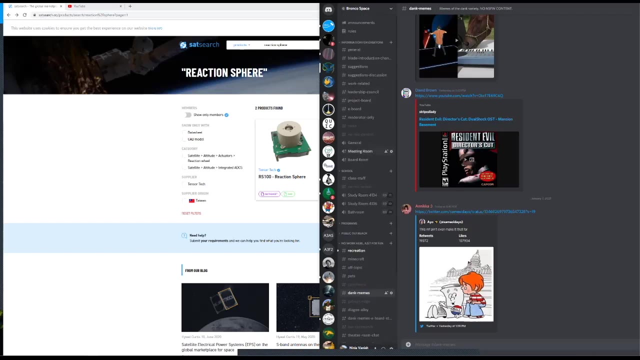 says that a 180 degree slew out of a beefy magnetorquer, it's probably going to be on the order of, like you know, a couple minutes right to complete that maneuver. um, actually, this is a great opportunity for me to go to the bronco space. uh, youtube channel. give me one second, guys, because 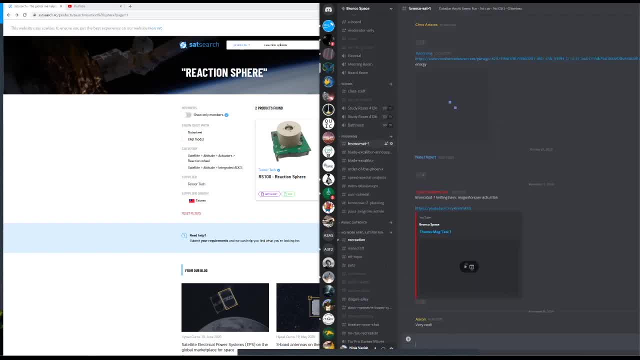 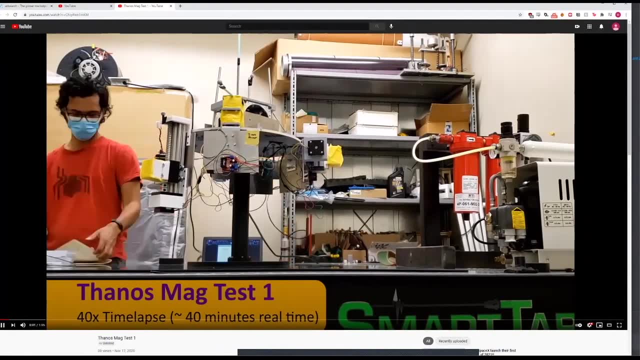 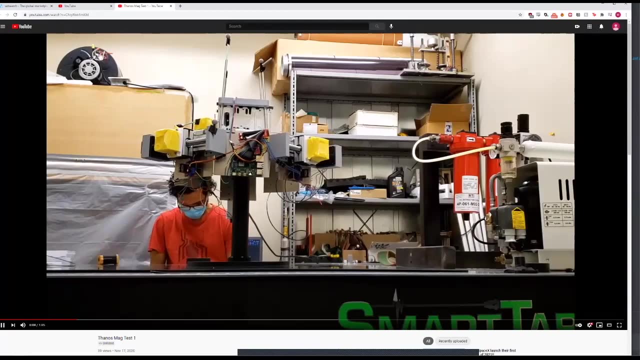 i just remembered we have a video there. is it here? it is? yeah, there, it is okay. so, um, this video that i have flashed up on the screen here, this is a 40 times time lapse, right, so, 40 minutes of real time. this is our satellite, this is a spherical air bearing system and, right now, the um we have. 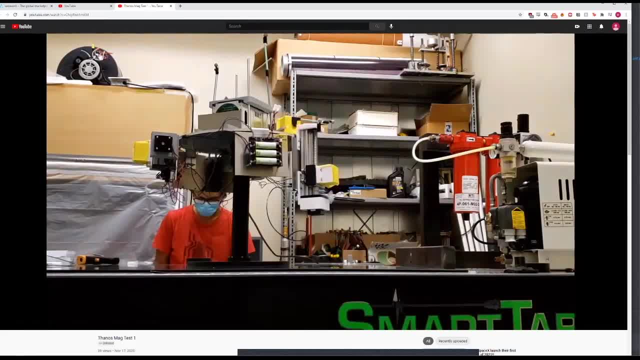 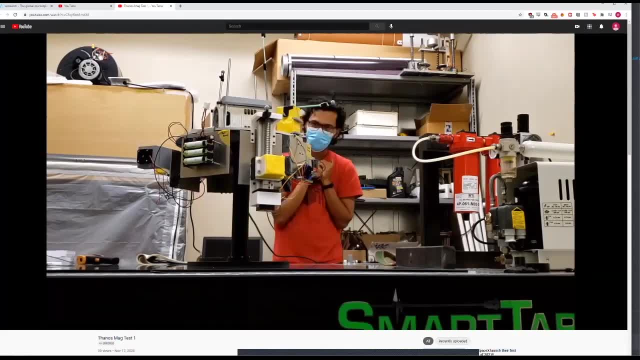 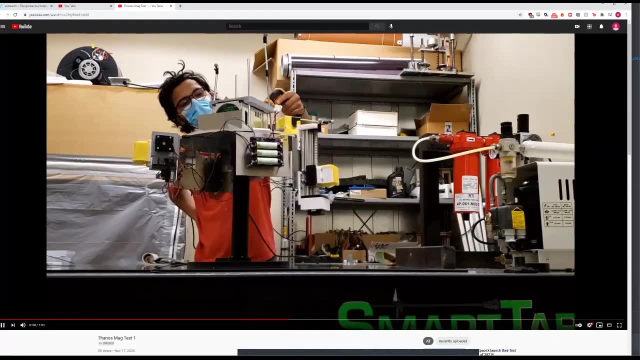 the magnetorquer going at full blast, right, and it is rotating. rotating the spacecraft- uh, you know, the spherical air bearing creates a essentially frictionless environment. now, as you can see, this is a 40x time lapse, so real time is like 40 minutes and not very fast. right like this is this: 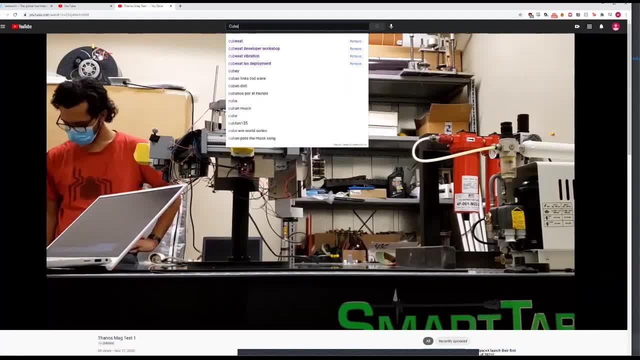 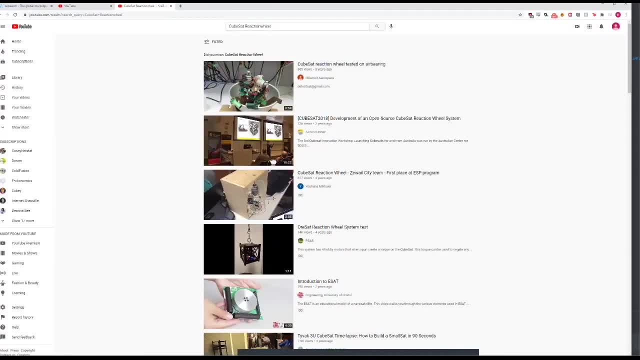 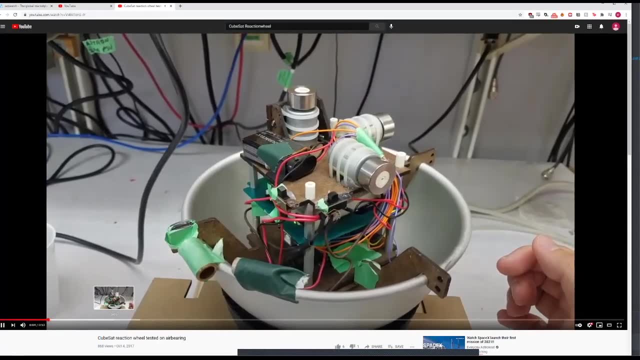 is not a speedy boy. um, on the other hand, you can actually just look up like keepsack reaction wheel, i think, uh, and it will show you something much more speedy. um, let me see if this is a good example. yeah, like you see that, you see the wheel turning here. 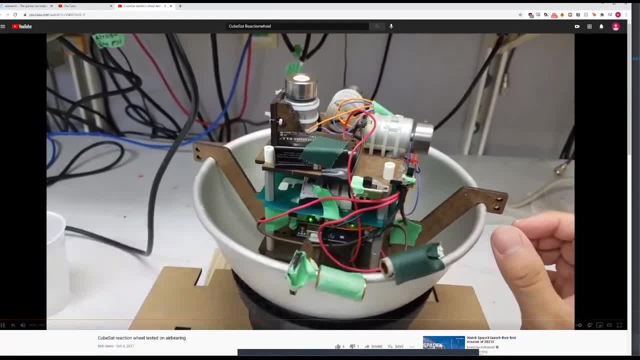 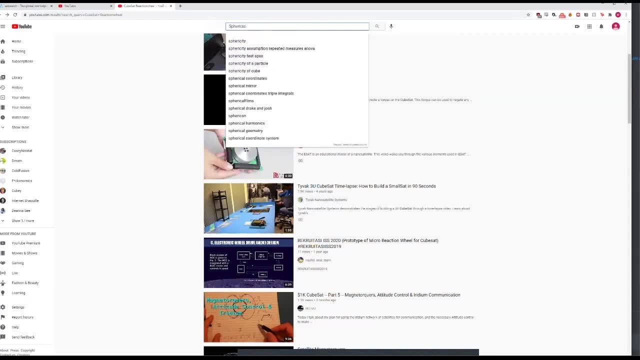 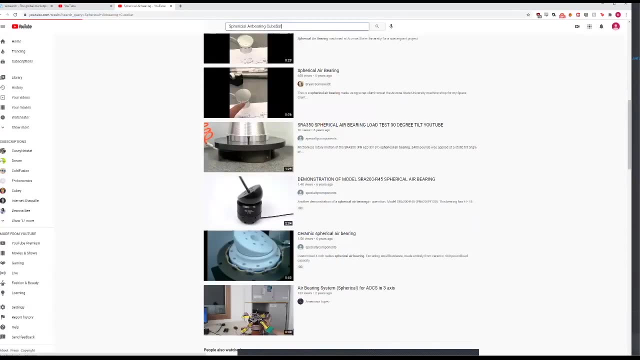 and this is real time, of course. so, okay, well, the guy's like bumping it with his hand, but, um, let me see, actually, uh, spherical air bearing. i think that's good, as you can see. i, i like it, just do it live. uh, this is a good video. 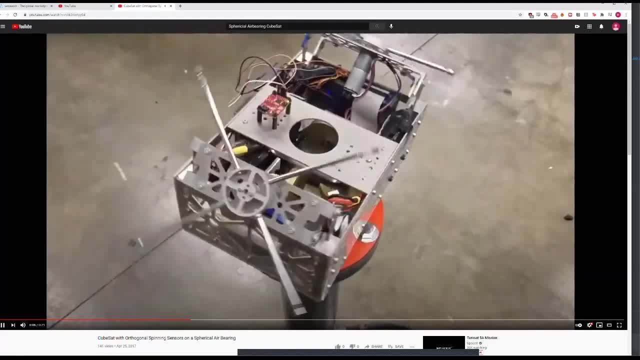 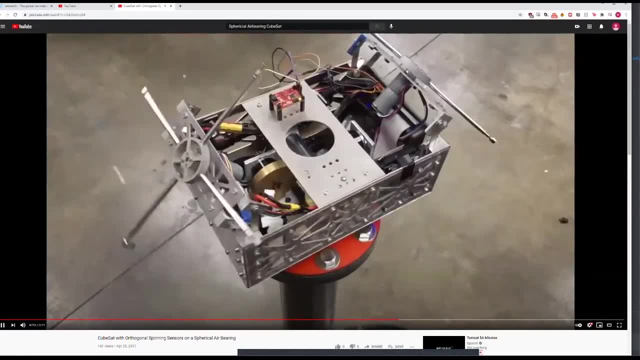 okay, i don't really understand the system going in here, but it looks like this is about a 6u size cube set with some really beefy uh reaction wheels in there that i assume are actually torquing on the system. yeah, so, uh, i would actually. 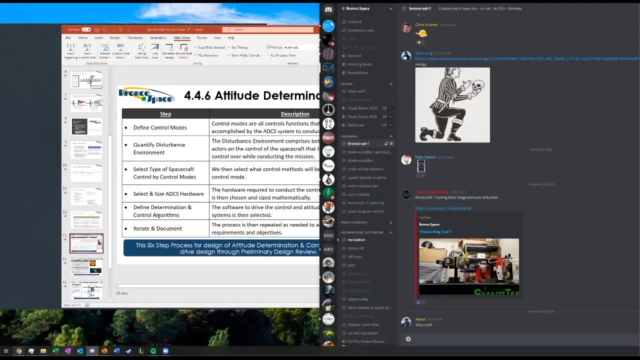 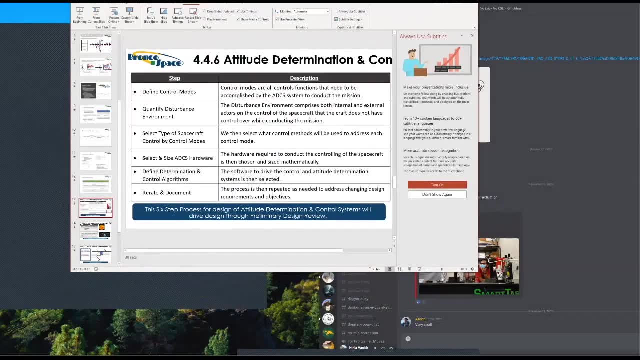 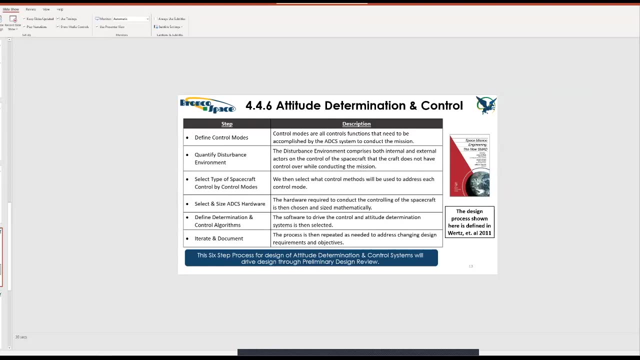 probably say it's fair to say that it is an order of magnitude difference in speed going from the magnetorquers to the reaction wheel. Does that sufficiently answer your question? Of course it depends on the size of both Beefy magnetorquers could theoretically generate more. 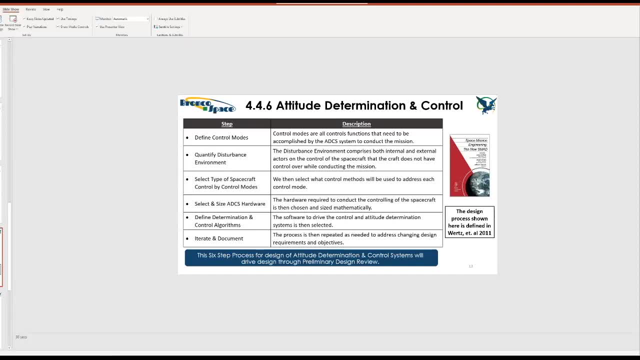 torque and move faster And at the same time puny. reaction wheels are going to move pretty slow But yeah, I would say reaction wheel completing a 180-degree turn in 30 seconds would be quick work And sometimes it can move even faster than that. 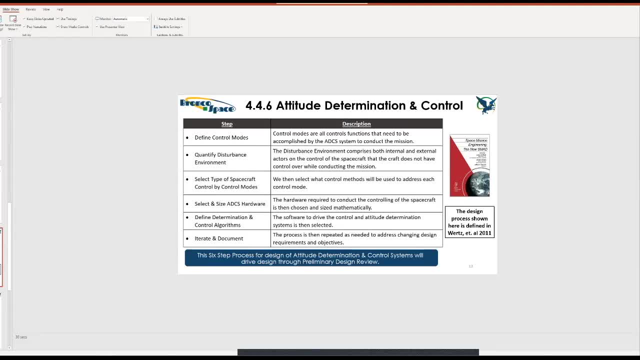 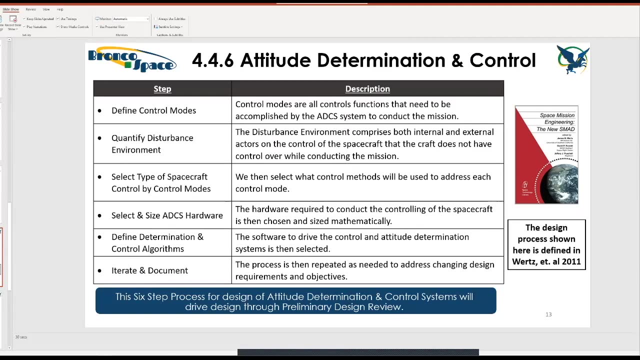 All right, Any other questions? Sorry, I was going to say earlier about the. I don't remember what it was called, but basically just the spinning ball that controls things. We're undergraduate developers. I feel like everything we do is a little sketchy. 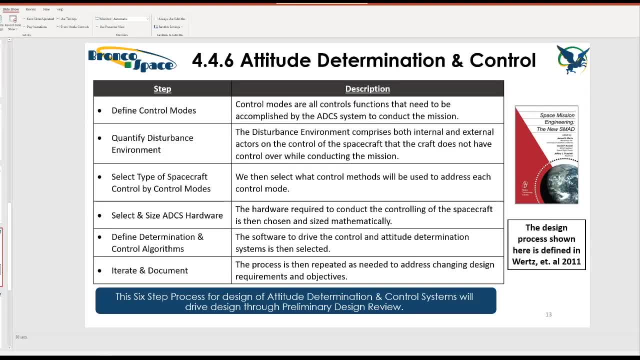 Yeah, No for sure, If there's time, I might even show what BroncoSat has cooked up, because it's a little Oh, Chris is telling me to, not, I think, Yeah, Yeah, One of our main problems that we're working on right now. you talked a little bit about it. 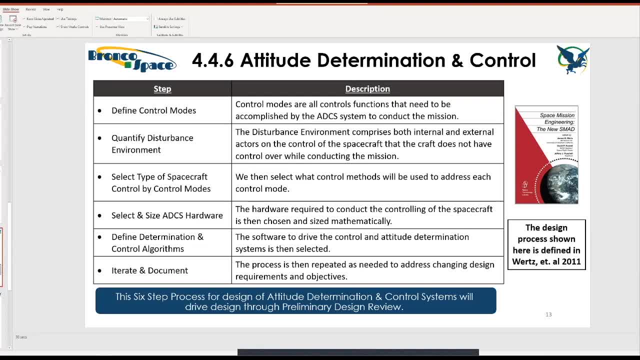 earlier. If solar panels are a big part of your design, you might want to figure out a way to point towards the sun all the time. So attitude control is something that we're determining whether or not we want a more, Just doing the permanent magnet that comes with. 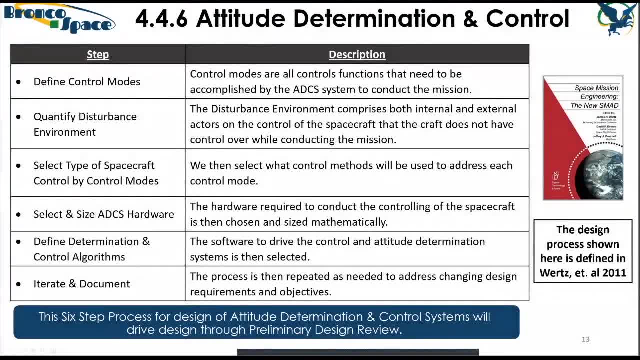 The fast bus or just getting an actual magnet torquer, And I guess I would like to hear your guys' thoughts on if it'd be worth it. Yeah, So my advice- as not a veteran engineer, but only a one-time CubeSat engineer- is: it's actually trivially easy to include a magnet. 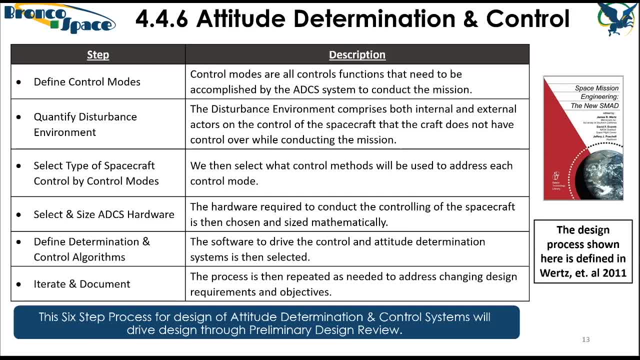 torquer in your system, As long as there's sufficient Foresight. If it's in your design from the beginning, then you can integrate one with relative ease, because it literally is just a coil of wire. We on BroncoSat have two torque rods and one open air coil, So the open air coil is 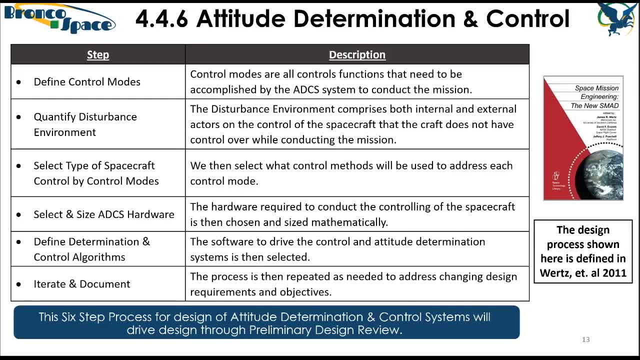 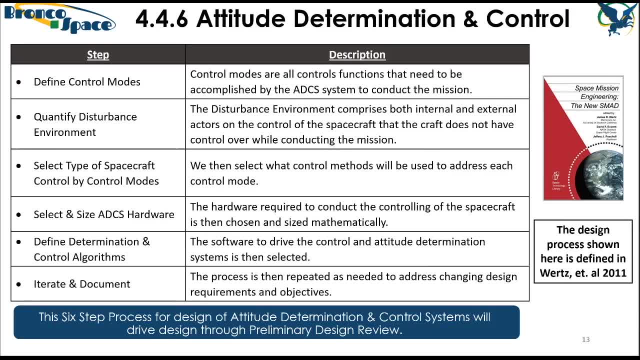 on a lot of different systems, and it's not just a small thing, right, It's a lot of different things, So we're actually using them on a lot of different instruments. Like we went to a commercial manufacturer and said: make us an inductor in this size, and they did it, And 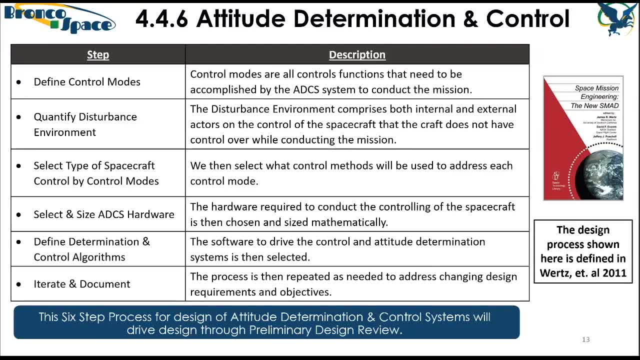 now we have magnet torquers, and we just have to run the current through them to generate them in their fields. The problem, of course, though, is that there is a lot of backend stuff that you need provide all the feedback for the system. 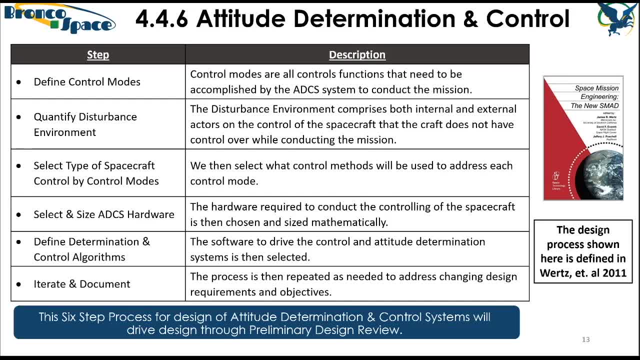 And then we also need to build out all the software to do the controlling, And that takes up a very significant amount of time and effort for the team. So you have to really think about it. Does it really add that much value to your mission? 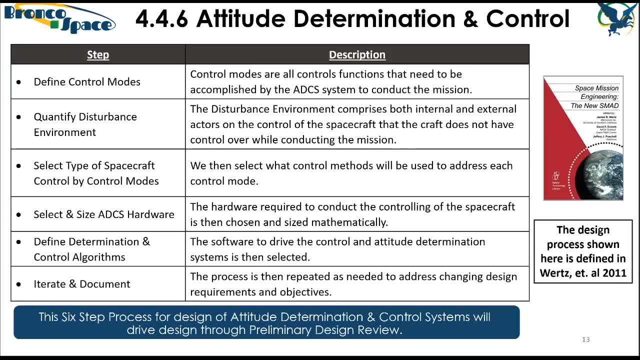 I think actually for most missions the answer is yes, But then of course you have to weigh it against like: is it a realistic thing for us to do? And the answer might be no in many cases where you're just trying to get something done kind of quick. 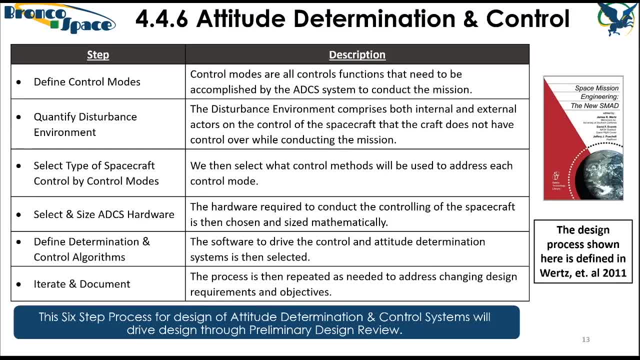 The engineering saying is, of course, never let perfect be the enemy of good enough. OK, thank you. Yeah, no problem. Any other questions at this stage? Oh, yes, OK. so why did you choose to use one open-air coil? 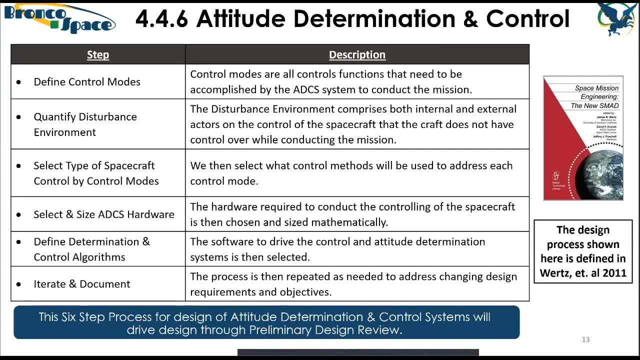 and two inductors as opposed to just three inductors? The answer is, that was the only way we get them to fit. The open-air coil is like this big: it's a bundle of wire, essentially in a circle or, in our case, a rough square. 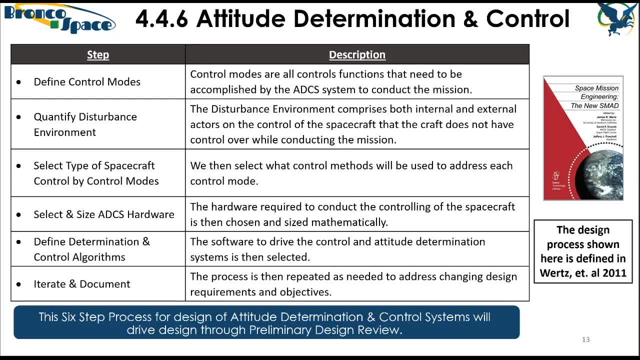 And so it's relatively flat. So if you remember right back to your electricity and magnetism- Yeah Class for us at Cal Poly, it's like 1520.. The magnetic field generated by electricity running through a wire is a function. 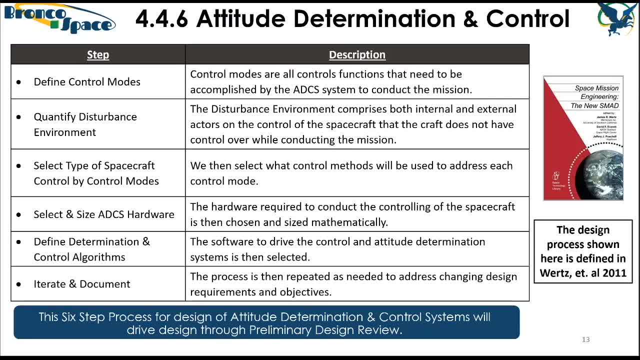 of the number of turns times. the current running through the NIA. Yeah, yeah, wait, Yeah, it's a number of turns times. the current running through the wire times the area enclosed by the wire. right, So you can move those knobs. however, 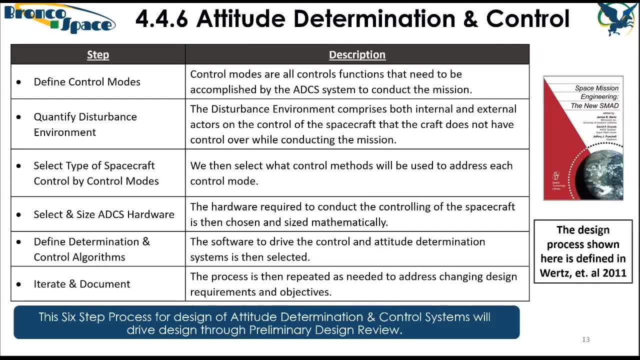 you please, in order to get the magnetic dipole that you desire. So when we have the inductors, there are a lot of turns. I think it's like 1,200 turns is how many turns we have on those inductors. 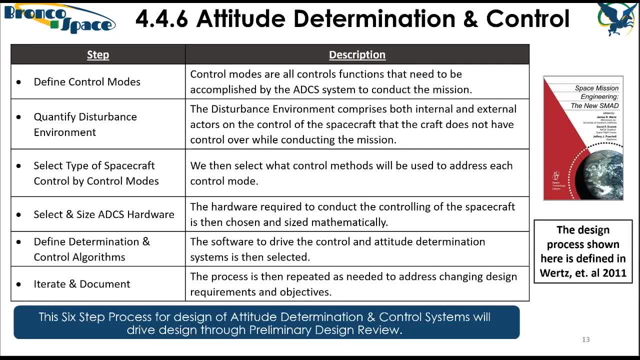 The current is like an amp, But the area that it encloses is not very big. It's like I don't remember how thick the bolt is. I think it's like a quarter inch bolt right that access the core. So the area enclosed is very small. 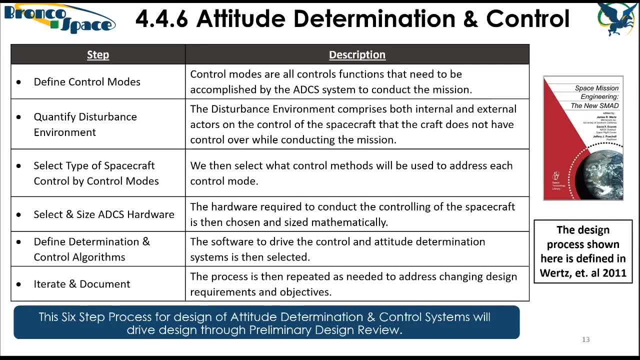 On the other hand, the open-air coil. it's only in the neighborhood of like 200 turns, I think, And the current is the same, But we are enclosing a much larger area, I think 50 square centimeters, with the open-air coils. 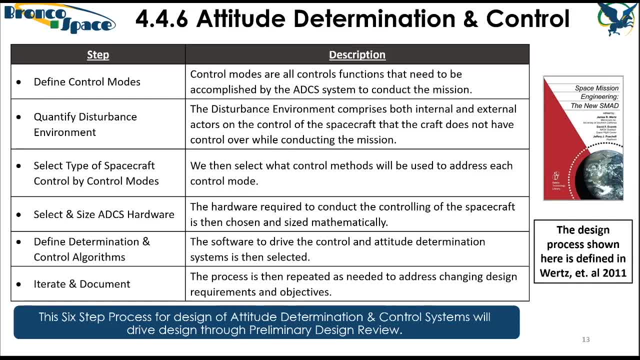 I'm probably less than that actually. So it's a balancing act And you have to decide not just what's going to give you the performance you require, but how is it going to fit in your system. In our case, we have these two solid walls. 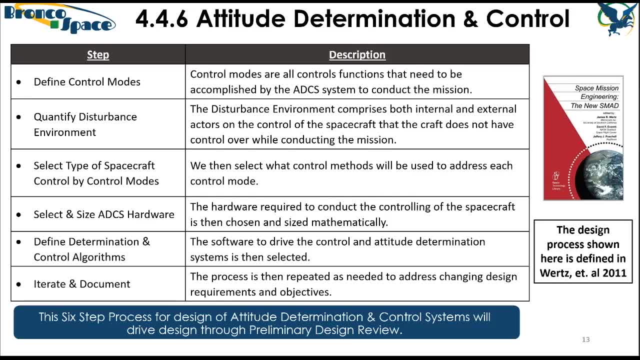 like six-sided cube. We had places to mount the MacaTorques 2 solidly on four out of six sides, But in order to get all three axes- the two sides that we did not have somewhere stable to mount a rod to. 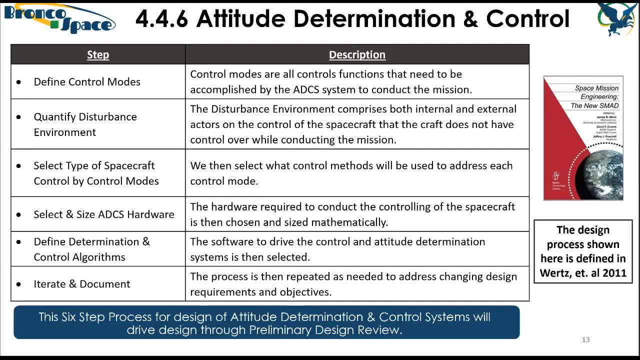 we decided instead just to have the open-air coil, because we literally just glued it onto the wall with space glue, And that's a pretty sufficient way to get around that. Yeah, Does that answer your question, Michael? Cool, cool, cool. 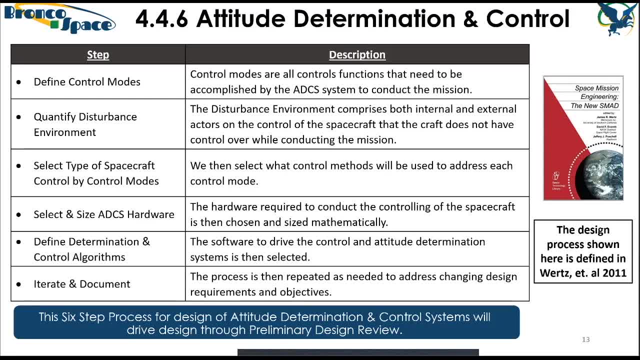 Any other questions? guys, Not all Soldier onwards. Take another drink of water real quick, Okay, So once you've selected your hardware- oh, I didn't even talk about the determination hardware. I'll talk about determination in a little bit. 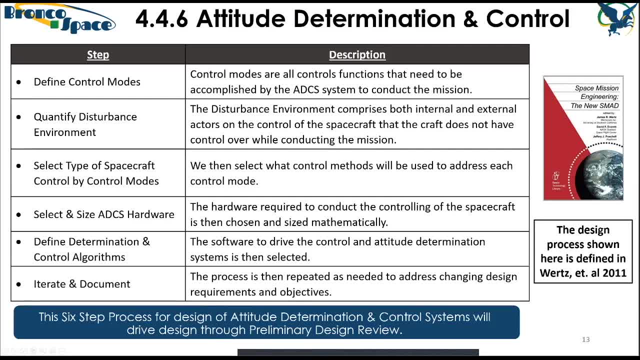 We'll just focus on control right now. Then you define the determination and control algorithms. So, like I said, it's not just the actuator you think about, It's also all of the software behind the scenes that makes the actuators go you have to think about as well. 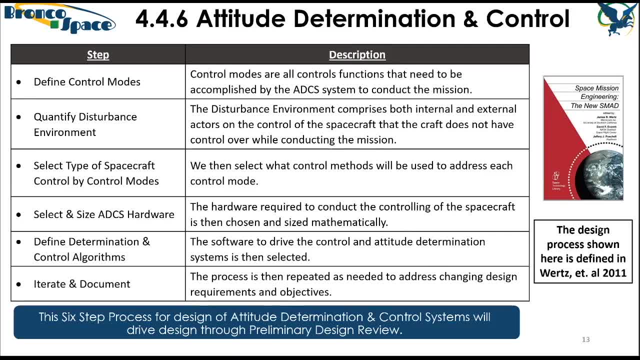 And probably the one that you're going to learn very quickly right in the CubeSat space, is this: it's a D-tumble algorithm from Magnetorkers, known as B cir is kind of what you think. it is, where you're basically taking the dot products. 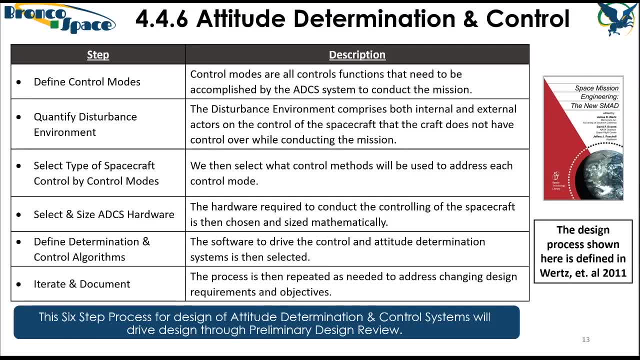 of the Ambient Magnetic Field compared to the magnetic field your spacecraft is able to produce, and you use that in order to get the difference down down to zero. right, like you, you're basically canceling out all of the rotational energy of the spacecraft until there's no, there's no change there. uh, relatively simple. 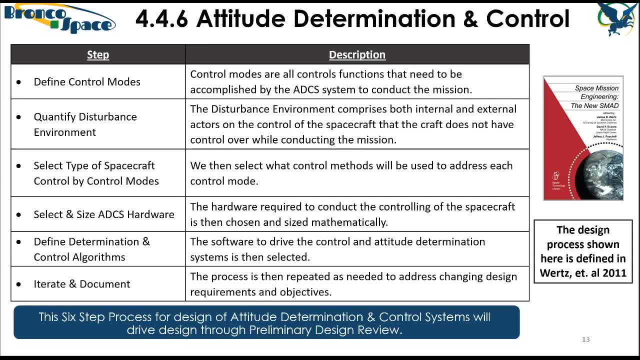 algorithm and, um, you know, if you need to do like pointing or something like that, that's where you have to introduce something like the pid control, right where you will have a targeted value, um, be it in like euler angles, which are your traditional, like zero to uh, i think it's 108, 80 degrees or. 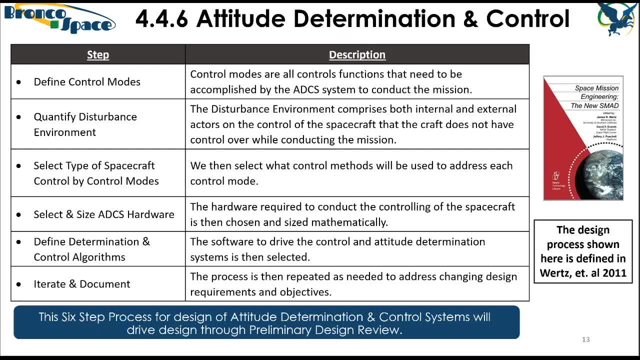 negative 90 to 90 degrees, depending on who you ask. uh, you have your euler angles right, or your quaternion, which is- um- i've had it explained to me- which is like a vector, but with more terms, so that it has, like state, information about the body as well. 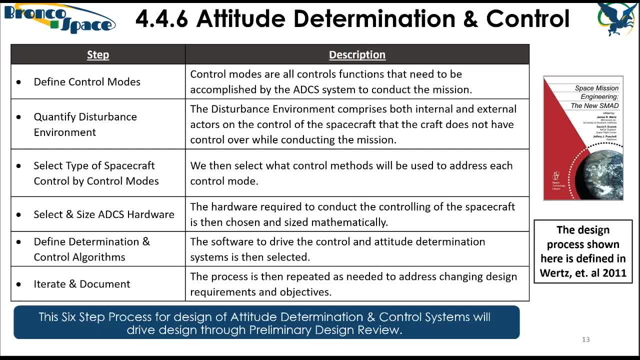 it's a vector that points in three-dimensional space but also has information that lets you figure out, like, what the faces of your object are. that's really kind of beyond the scope of this like introductory workshop. but euler angles or quaternions right are the two sort of 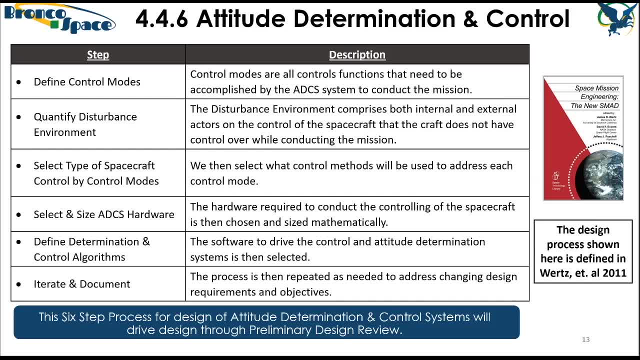 possibilities you have for you know your control input, like go to this euler angle right or go to this quaternion, um, and then the algorithm is what actually moves the spacecraft there, um, yeah, and then, once you sort of figure this stuff out, it's very important to iterate and 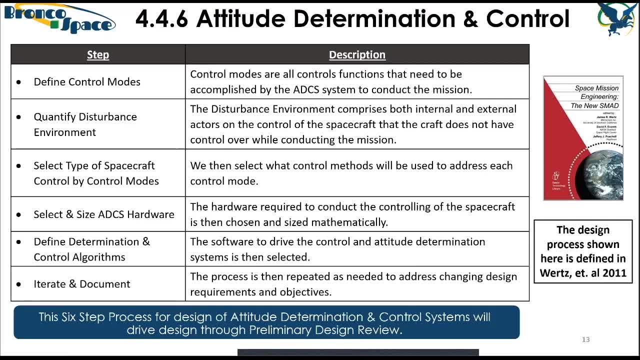 document this process right? uh, it's very rare that like first, right off the bat, you're going to figure it out right away, like for bronco set. um, you know, we had like an original torque rod design right that we went to test and then it just didn't really work as well as we wanted it. 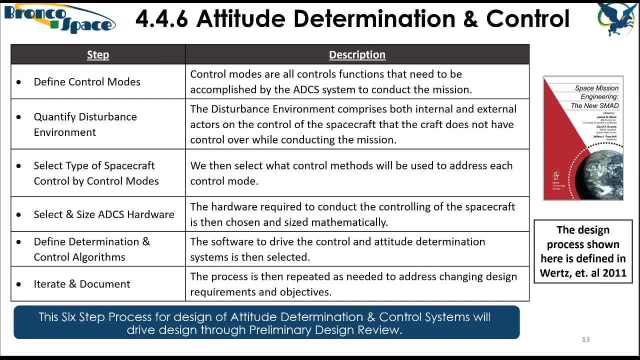 to work, so we had to beef it up at more turns right, um, and then we had to figure out how to? um. we also had to, for example, like um, mess with our motor drivers in order to actually get them to perform the way we wanted to. um because the interface between the motor drivers and our flight 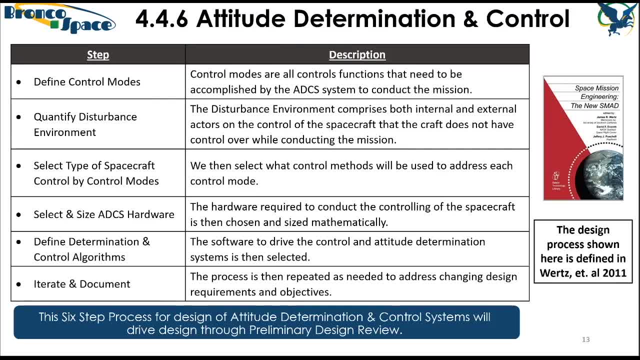 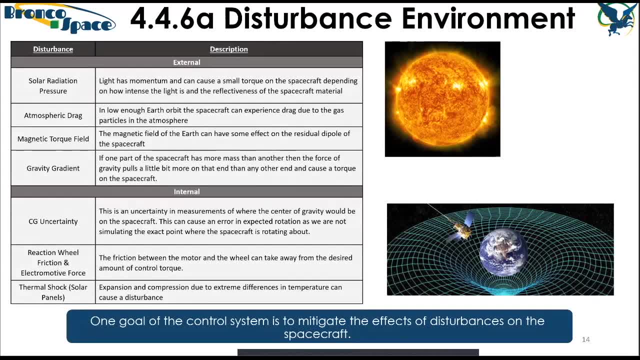 computer was kind of wishy-washy right and, um, yeah, there was a step by anything i could do there. so here's the disturbance environment. i was talking about how much open source software can be reused. um, i think there's actually a pretty decent amount of open source software out there. uh, i know that. 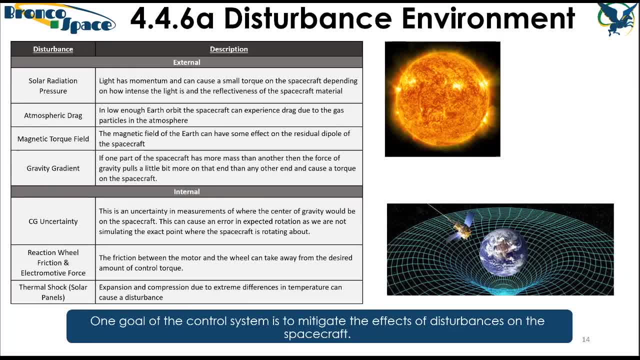 like um b dot, for example, is such a commonplace algorithm that uh, you can find like b dot source code just kind of floating out there, uh relatively easily. and also, like looking into like research papers, you can find a b dot source code uh just like a dependent to the end of research papers. 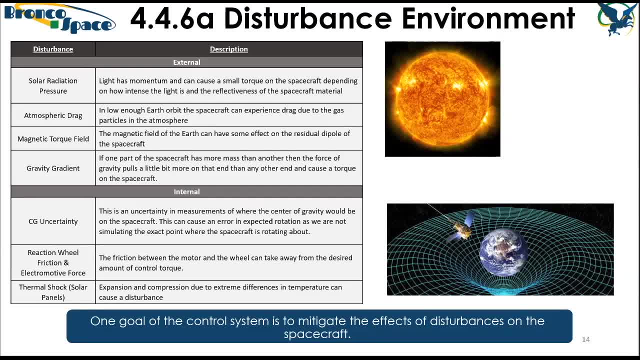 the. the issue, of course, with open source software is that, at least to my knowledge, uh, there isn't really sort of an end-all, be-all like software solution, um, because every satellite is different and um, okay, let me, let me just like quickly backtrack real quick so y'all remember back here, right where, 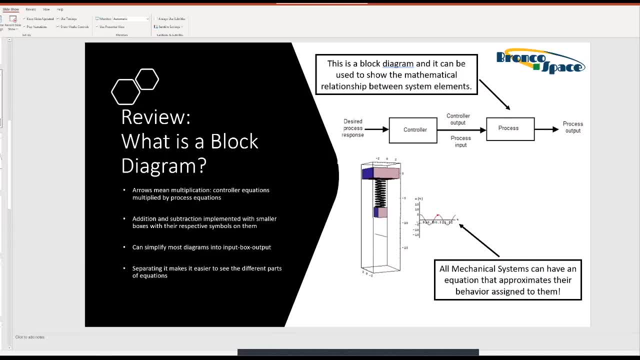 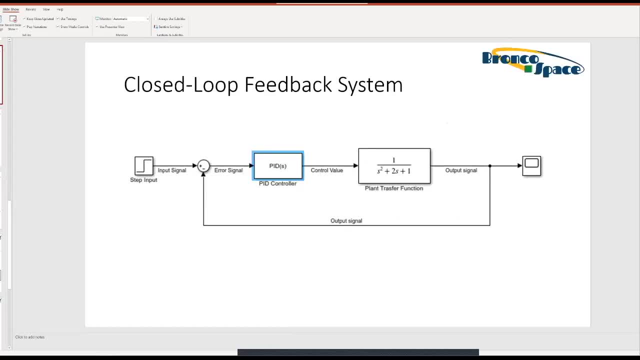 we were talking about, like you know, block diagram and like the, you know the plant right and all that stuff. so when you have um, when you're, when you're designing your control system right, like the, the gains, for example, that you stick in your pid controller, these are always going to be different. 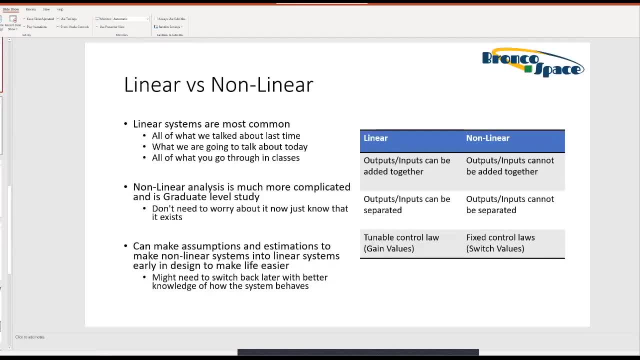 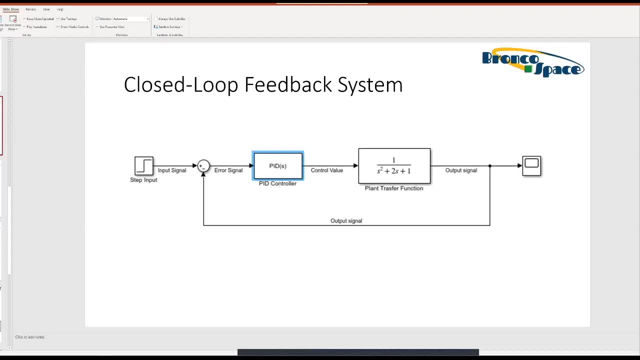 depending on what your system is, um, like. let's say, like you know, you have like a really heavy spacecraft right, um the you. you can't just copy and paste like another control system onto that control system and expect it to work right, because if you, if you take code that was meant for like 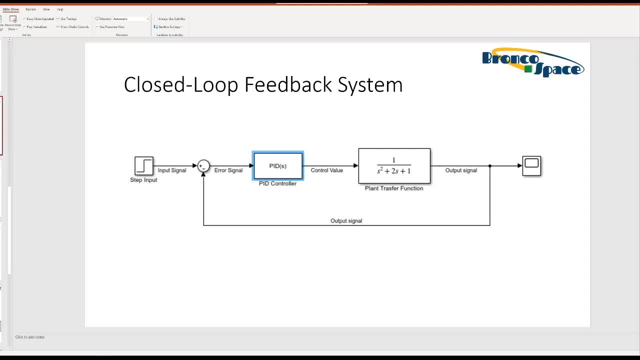 you really like spacecraft and then impose it onto a heavy spacecraft. well, most likely, what's going to happen is going to be: it's going to be like way under, uh, like, like, like uh way. it's going to way underperform, right, because it just wasn't designed. 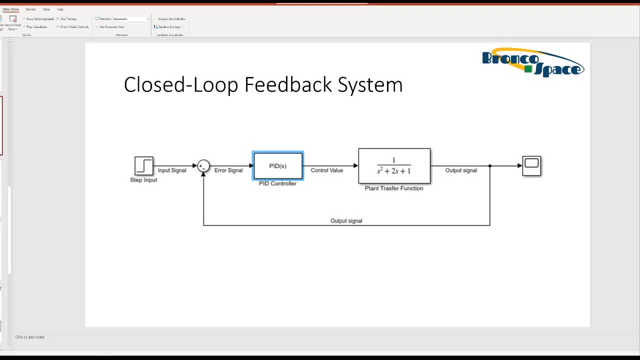 to be like a heavy spacecraft, right, so you can't just copy and paste like another control system to work with that system. um, this is sort of like a enduring problem, like uh with um, with like just space mission engineering in general, where because every satellite is kind of designed like to spec, 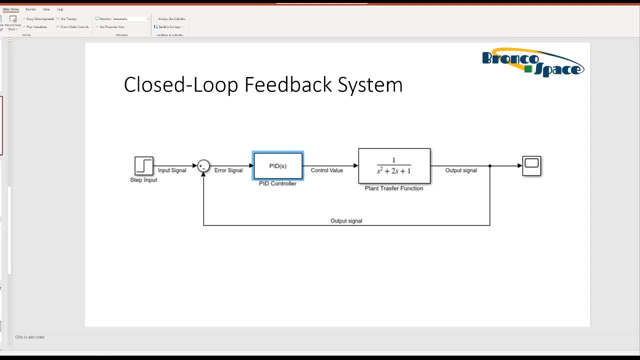 and in a way that it's like we're just trying to meet, like the specific mission requirements that are set out to us. um, it's hard to sort of just transfer, uh, like something that worked over here, we're just going to put it over here and expect it to work the same way. um, one of the sort of the 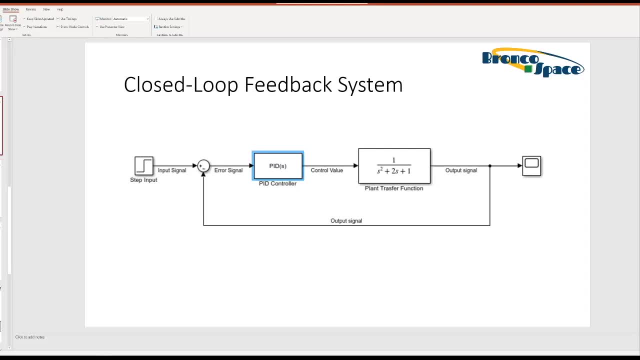 up-and-coming sort of uh things that might make this a lot better is actually the uh use of like artificial intelligence or machine learning to have a control system, sort of like tune itself. because usually what, when you actually get down into the weeds of it, what usually has to happen? 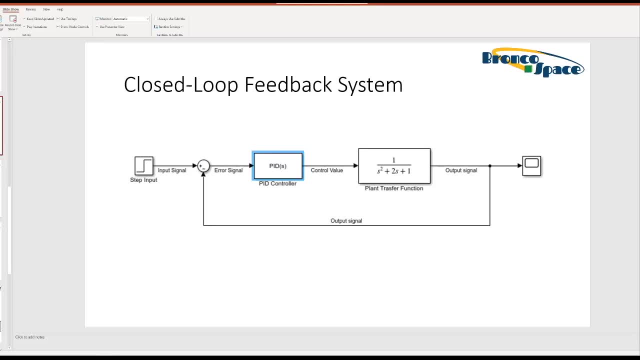 is that you, like, as the engineer, have to simulate the system, observe the system and see. oh, you know, it's moving too slow right, or it's oscillating too much. uh, why don't i manually turn these knobs right, and then we will get a result out the other end. 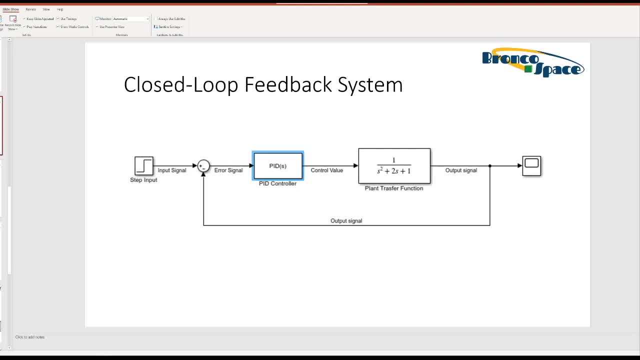 or you know, if you have fancy pan software, the software can kind of do that for you too, right where the software will just randomly turn knobs until it gets to like a desirable result based on your requirements. um, one of the up-and-coming fields is like the use of like an artificial. 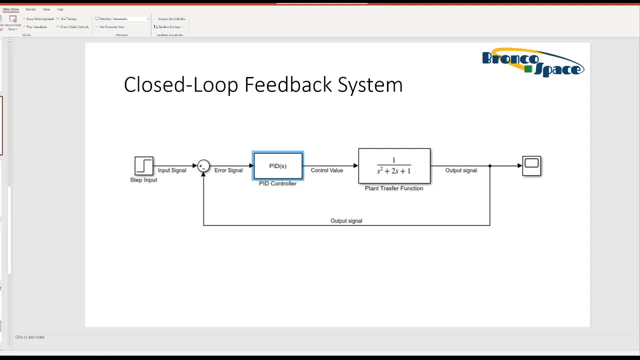 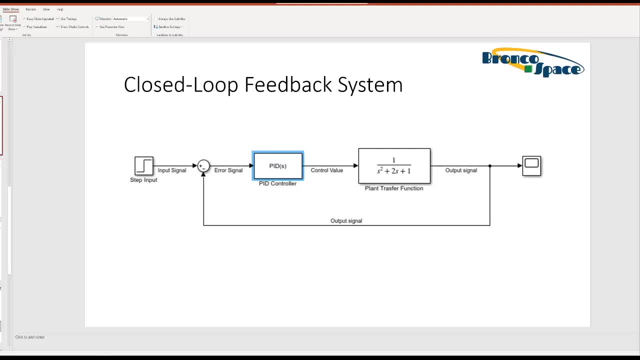 to exactly everyone's preference. but you, as a human right with your brain, you can figure out how to tune yourself right in order to drive the car effectively. uh, same sort of idea with the satellite right, where one day, maybe, we can have the satellite teach itself how to. 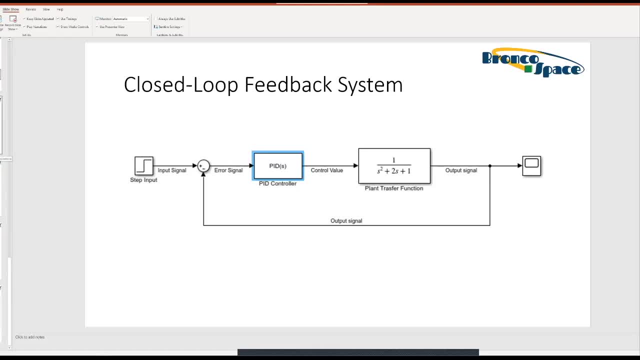 how to do all that. so that was a really long-winded like tangent. i just went on there. uh, does that answer your question? kevin, i totally. i could have just said there is software and it's not really that reusable, and that would have probably answered your question. um, yeah, yeah, that helps. 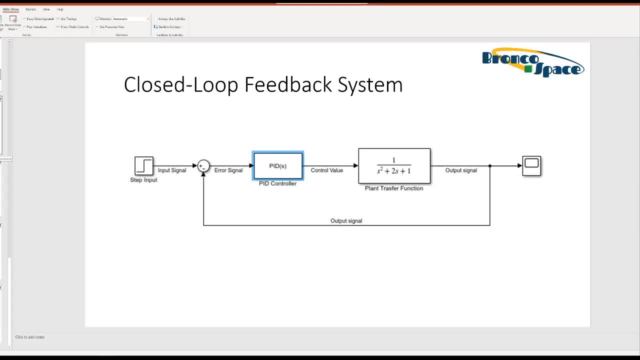 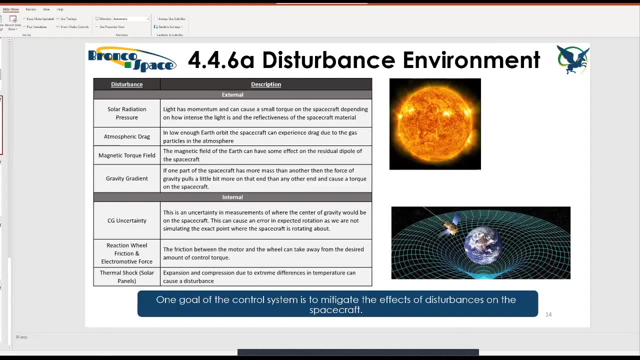 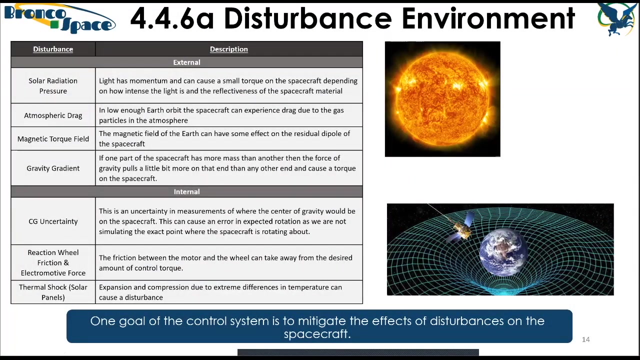 thank you all right. yeah, i i sure wish we could just copy paste stuff off the stack overflow for this, but it's a little more nuanced than that. okay, yeah, so this is the disturbance environment. um, i'm really just winging the flow of this year, so you have a whole lot of things that can contribute to like things that will disturb. 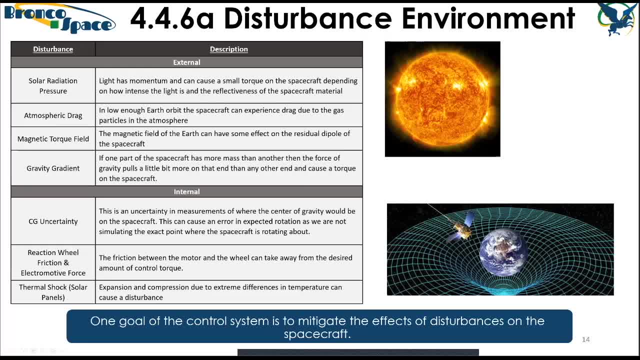 your spacecraft, um, like radiation, pressure, drag, magnetic, torque, gravity gradient, um, and the interesting thing is that you can actually use these disturbances to your advantage as well, um, for example. um, there, unfortunately, you'll have any. i don't have any naval academy folks joining us for the hackathon, but a couple years ago, uh, one of their cubes. 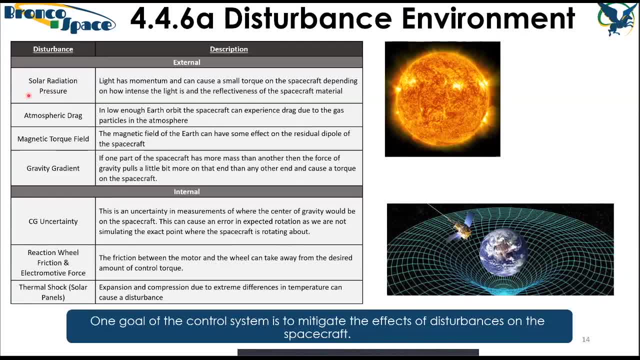 assets that they flew actually used solar radiation pressure as a control method, rather than like a magnet worker or anything like that. uh, what they essentially did is they painted half of their satellite in a bright white color and the other half in a more dark kind of black. 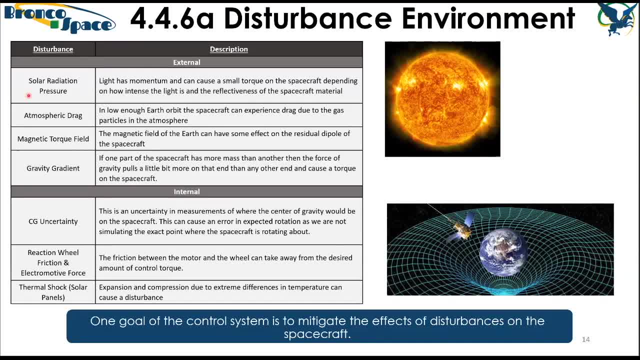 And what that created was a mismatch in reflectance, right, So that the solar radiation bouncing more off of the white side of the spacecraft actually induced a spin on the spacecraft and they achieved spin stabilization purely based on solar radiation pressure. Maybe more famously, you know, some engineers are trying to develop things like light sails, right, You might have heard of light sail and light sail 2 from the Planetary Society, where they unfurl this massive mylar blanket in space and then just the photons bouncing off of it generate a force that will, that can, over time, you know, speed up or slow down a spacecraft. 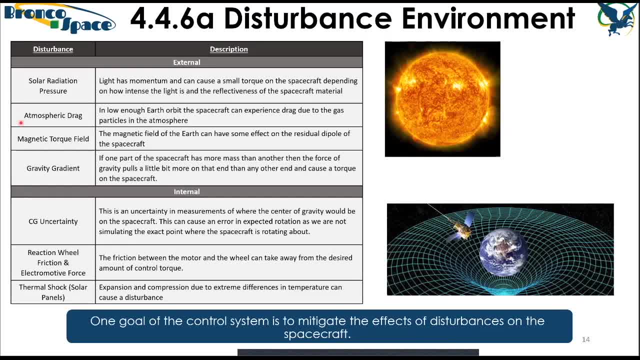 I guess for a drag just kind of, is a drag Like it can sometimes be used as a control method, Particularly like you can use the drag to orient your spacecraft in what's known as, like the ram direction. but using atmospheric drag is usually not really something that is ever designed for, because it's highly inconsistent once you're in orbit, because atmospheric drag turns out to be at the incredible altitudes of space. 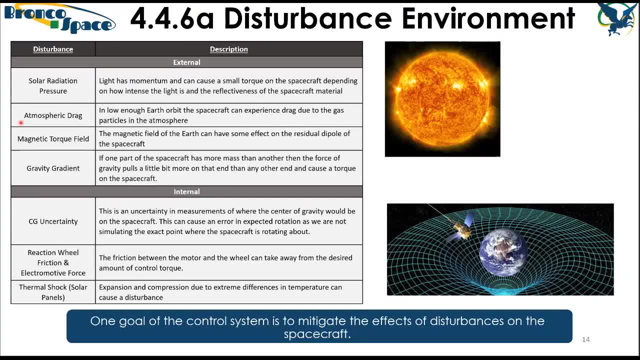 Entirely dependent on solar activity. when the sun hits the Earth more vigorously, right, the atmosphere actually expands and creates more drag. Right now we're in a legendary solar minimum, so there's actually very little atmospheric drag to work with. I already talked about magnetic field. 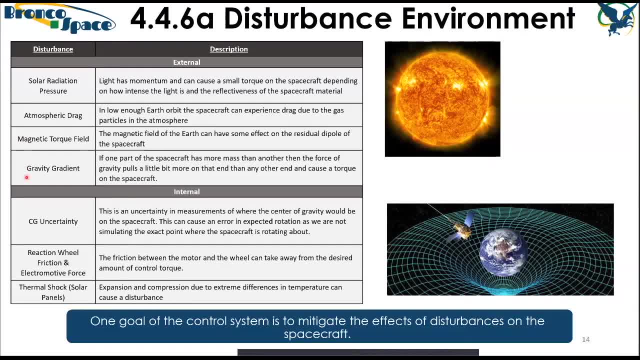 Gravity gradient is something that a lot of big satellites use. pretty often, CubeSats have tried to use gravity gradient, but to my knowledge, there has been no CubeSat that has successfully used a gravity gradient control method, mainly because, like they're too small, Like there's not enough mass there to work with. The premise, though, is that if your spacecraft is very 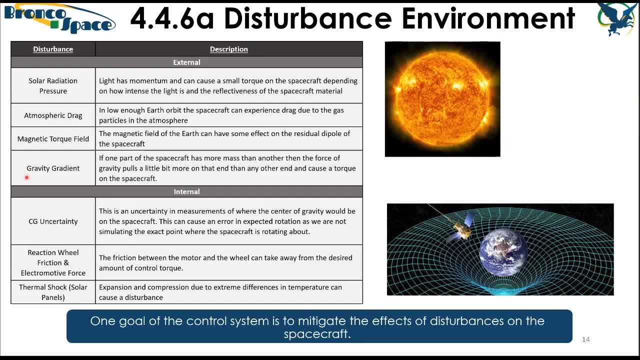 lopsided in weight to one end, the heavier end will want to orient itself towards the Earth. Imagine kind of like a pendulum, right like the heavy end wants to point down towards the Earth. Unfortunately, like again, CubeSats are kind of too small to really use gravity gradient, but some people have tried and unfortunately failed. If you want to look up the Firefly satellite, I think that's the most like famous example of that. 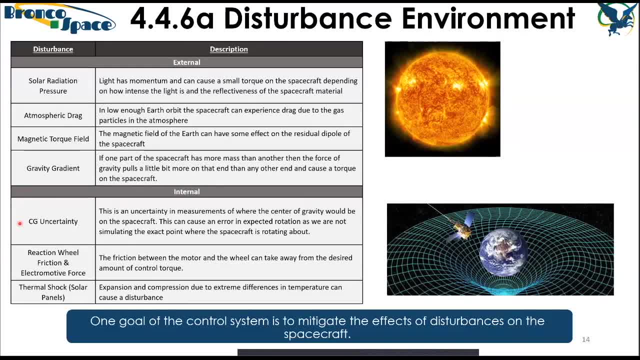 There are some other sort of internal disturbances we're into too right, like CG, uncertainty, right. This isn't a huge problem for CubeSats, actually, because usually CubeSats aren't losing mass while they're operating like there's no propellant that's being burned or anything like that. so 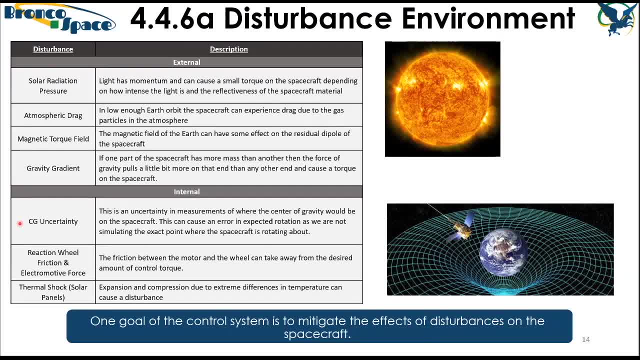 if you get a good CG on the ground it kind of sticks. Big problem with reaction wheels is that they generally will experience friction right, which over the life of the wheel will introduce a small disturbance torque And, more importantly, can also sometimes induce failure in the wheels, which just leaves you totally shit out of luck. 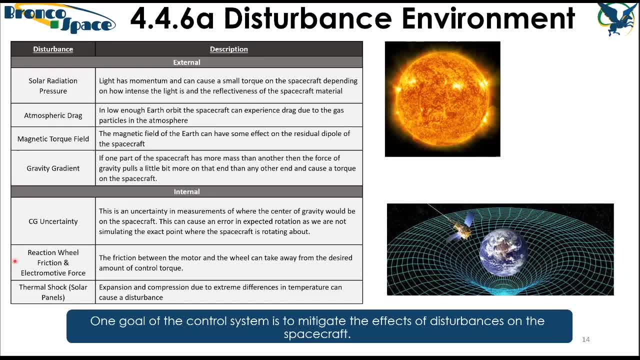 And the other thing with reaction wheels is that they can actually saturate, which is essentially when the motor is spinning so fast it cannot spin any faster, And at that point you just run out of control authority, right. like the motor cannot speed up anymore, you can no longer, you know, induce more, more torque. 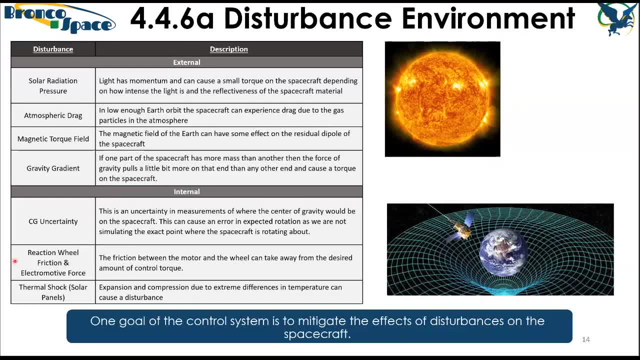 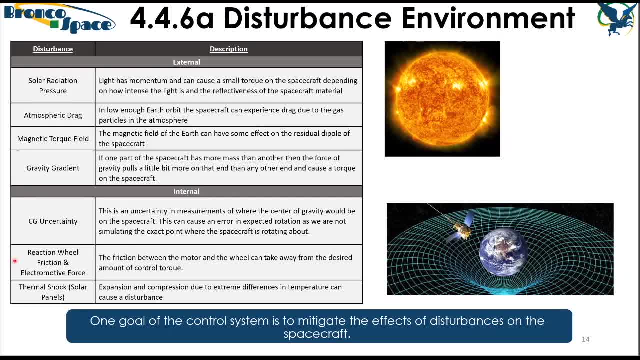 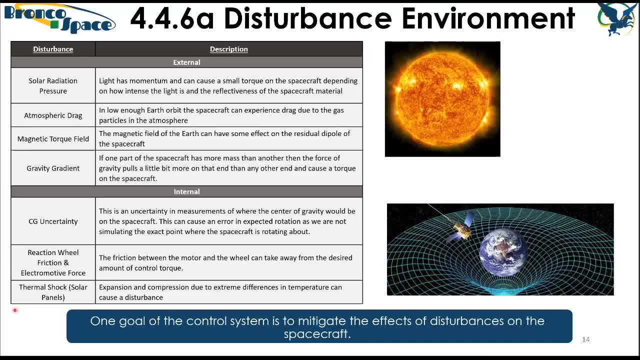 rapid thermal expansion that happens as a result of the sun suddenly hitting you know the cold and dark spacecraft. can you know introduce like a little jolt that can be an issue for really, can be an issue for really. 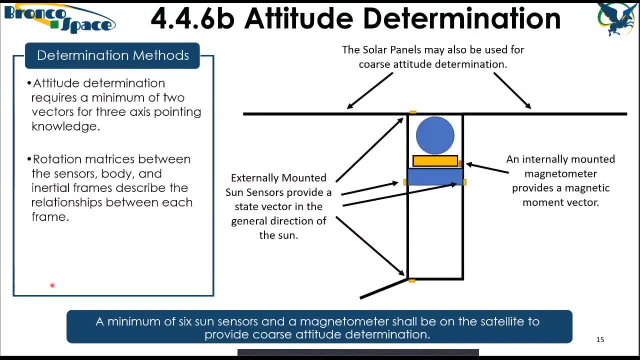 sensitive missions. So here's actually an example of what a really high level design for a ADAC system might be. Here is an amazing PowerPoint sketch, using PowerPoint auto shapes, where we have noted that there are externally mounted sun sensors. So this is where I need to acknowledge 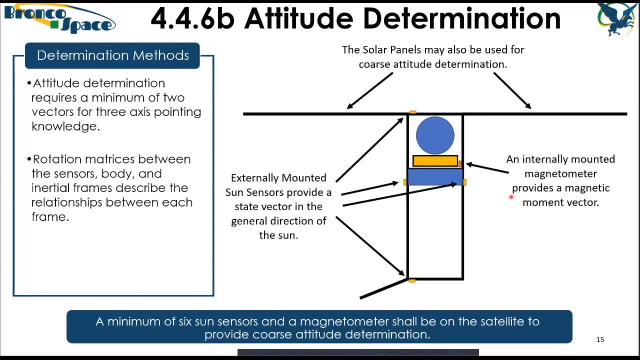 that there's also a determination aspect to attitude control, where the spacecraft needs to be able to figure out where the spacecraft is And, more importantly, it needs to figure out where the spacecraft is pointing, because the spacecraft does not have eyes. And then 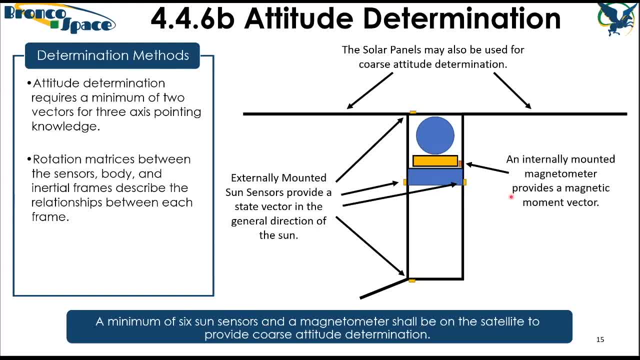 in the cold darkness of space. there's no reference points. Robot arm is just bolted to the ground. Robot arm knows where. robot arm is pretty much all the time based on its original location. But when the CubeSat comes out of the deployer, 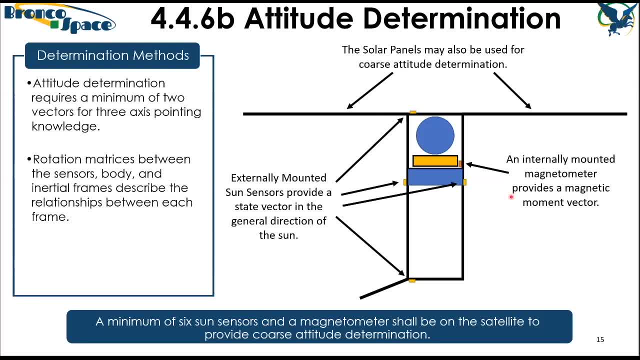 it will essentially have no knowledge of its surroundings or its initial state And, as a result, it needs to use external sensors or internal sensors to figure that out. Pretty commonly you'll see magnetometers inside satellites. Pretty much all satellites will have a magnetometer. 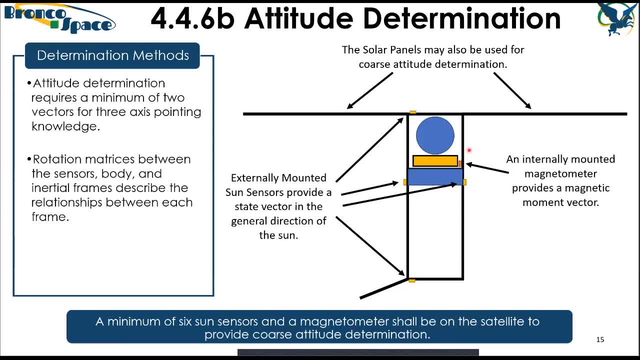 And, on the other hand, that's pushing the satellite to steady detective positions to observe weather, taking mournful pictures, leaving its GPS and recording data and all of those things being communicated to – when you're outsideыми, there's a magnetic field to get an understanding of where you are relative to Earth, And most, if not all, satellites will also have externally mounted sun sensors in some way, Because these can provide a state vector in the general direction of the Sun. The premise here, basically, is that you can understand where the sun is in space and then locate your satellite. 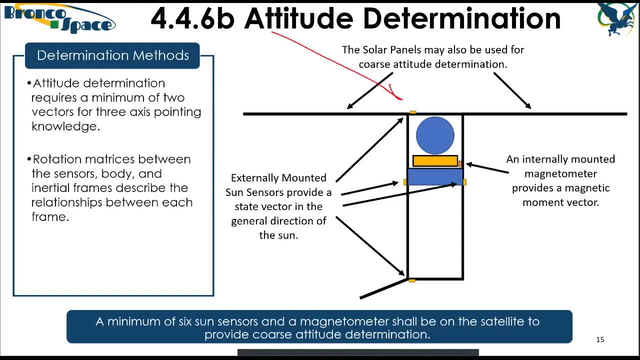 using that. where you have sun coming in like this, It'll only trigger these two sun sensors. So therefore, the sun is in this direction and obviously not in this direction, And you can also use more advanced sensor fusion methods to really actually provide a shockingly accurate orientation. 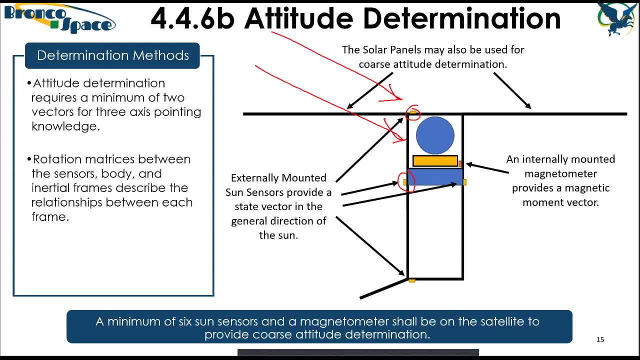 for your satellite based on these sun sensors. You can also use the solar panels. So here I've noted that these are dedicated sun sensors which might manifest as a UV sensor or a photoresistive sensor, But some satellites will actually just 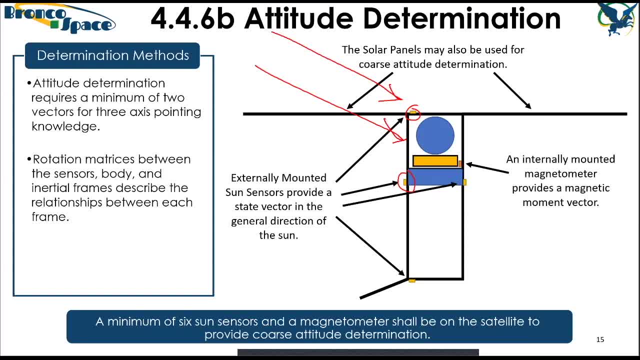 use their solar panels because depending on the angle of incidence, that is, the angle of the sun relative to the solar panel, So the voltage or current depends on how they're wired of these solar panels- will vary And you can take, you can develop a model basically. 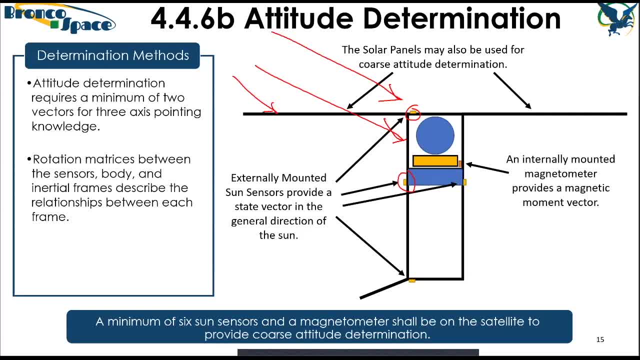 where you use the varying currents and voltage in the solar panels, exactly as you would use the varying currents or voltage in your dedicated UV sensor or photoresistive sun sensor. Yeah, So those are some attitude determination things. I know Stanford Flynn had to jump out. 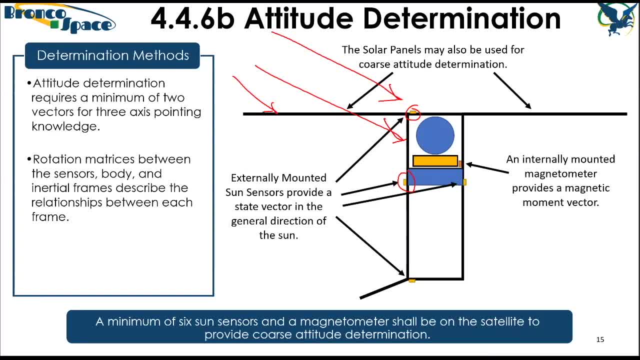 to eat dinner with his family. But Stanford they're trying to have an AI actually figure out the attitude of the satellite just by looking at pictures that an outward-facing camera takes. So that's sort of like a new frontier New frontier sort of technology. 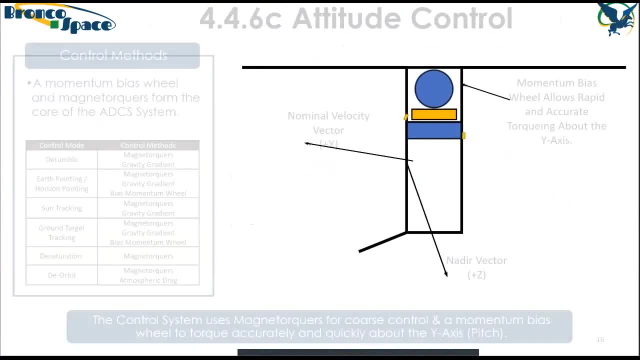 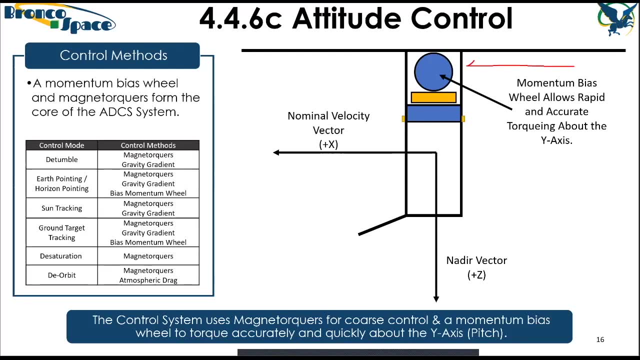 Yeah, Now also on this design, if we kind of go to the next slide, we also have some control stuff here, right, Where, like this 3U satellite, we have a momentum bias wheel here, right? So this is imagine just like one reaction wheel, right. 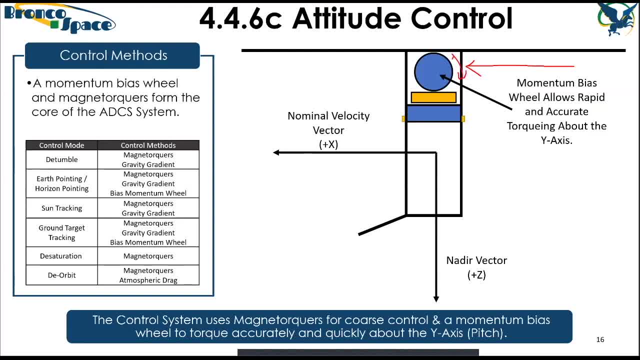 Like in this axis, And so if it's spinning this direction or the other direction, it can induce a torque about the. I don't know about the y-axis, assuming that the y-axis is coming out of the page, And why you would want to do this is well. 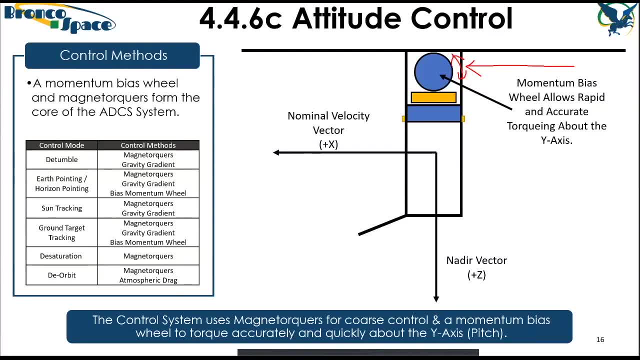 one reaction wheel is less complex than three reaction wheels, And for a satellite like this, the example here is that this is an Earth sensing system. Imagine this is a camera in here And you want to maybe track position on the Earth, right? 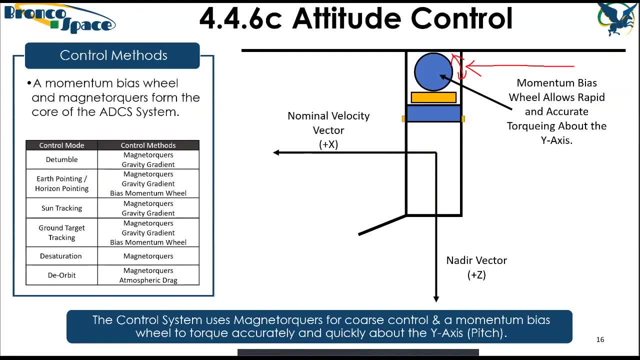 Magga-torquers don't have enough, Yeah Yeah, They don't have enough control authority to do that rapidly. They can't make that relatively fast motion to track an object as it flies under the satellite, But a single reaction wheel in that axis. 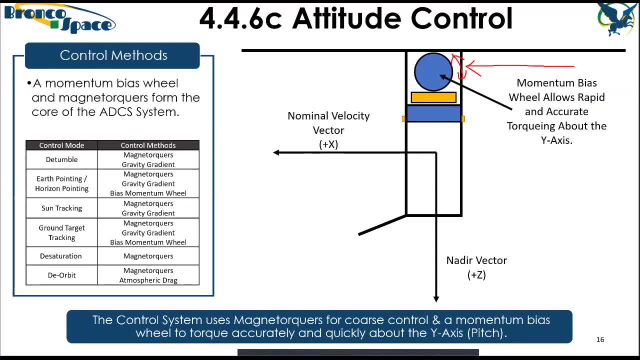 can actually provide that push rapid slew, as it's called, And then you'll have magma-torquers just for controlling the other axes at a much more leisurely pace. Yeah, Oh, Here's just some nomenclature, Right? 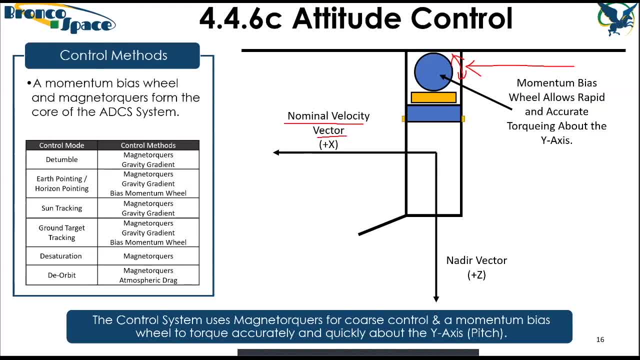 Like the velocity vector right by convention is usually positive x right. That's the direction the spacecraft is traveling in. And then the nadir vector: nadir is directly down right. So imagine a line that just goes straight down. 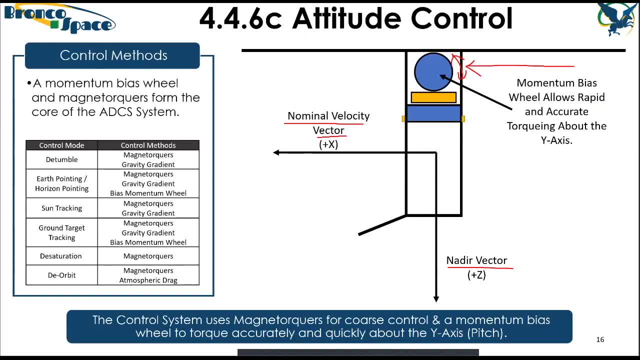 from the satellite into the planet And then zenith- right, if you encounter the word zenith, that is directly up right, So straight out of the satellite right, Straight out of the planet, directly up through the satellite. Here I've also noted some example control modes. 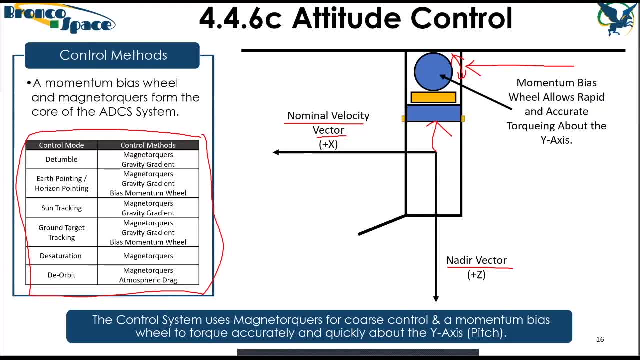 and then the control methods associated with them. So, for example, when we come out of the deployer right, there's an unknown amount of spin that is put on by the whole spring-loaded box thing. So we need to de-tumble with our magma-torquers. 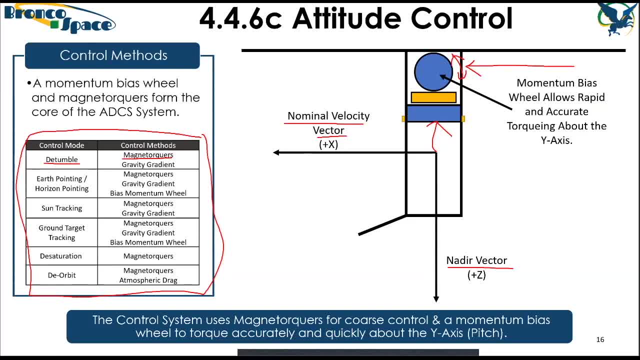 and a little bit of gravity gradient helping us out in order to stabilize the spacecraft, Then, right, We might need to do some earth pointing or horizon pointing to sort of orient the spacecraft, get it ready for doing imaging or things like that. Then we might have like sun tracking right. 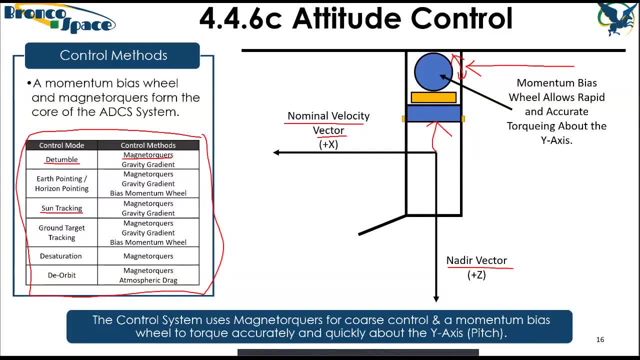 If you have, like these, deploying solar panels, we need to charge the spacecraft up. We'll want to make sure they're pointed so that they're perpendicular to the oncoming sunlight so they generate maximum power. There might also be like ground target tracking, right where 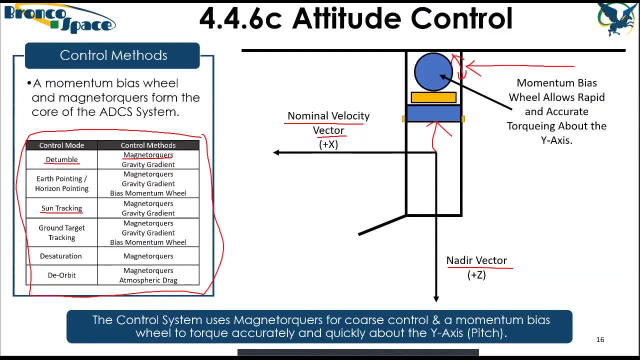 you know we're flying over a ground target and we want to maintain a fix on it as we fly by, so the camera has a lot of time on target. There's also just desaturation, right, Because, remember, those reaction wheels can get saturated. 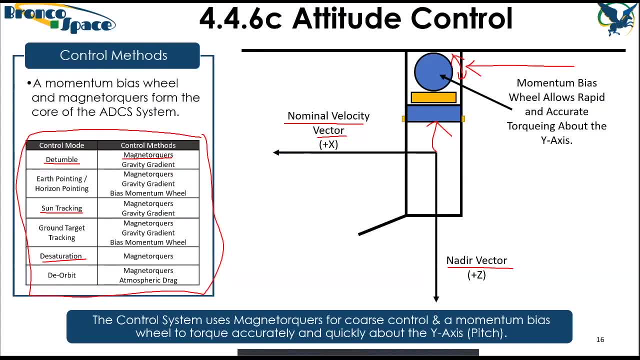 You want to make sure that you're able to desaturate them. so you know you can still get that rapid maneuvering, And deorbit is actually a control mode that I think most CubeSats do not have a like. do not implement something for. 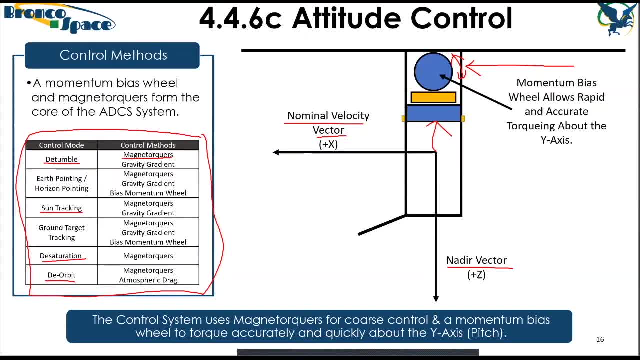 but it's good practice to also have a deorbit control mode Where, if it is like all possible, you try to orient the spacecraft in the way where you maximize the cross-sectional area of the spacecraft And what that does is it increases the drag. 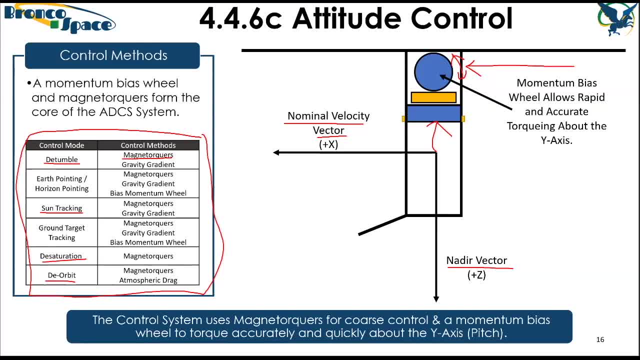 and causes the spacecraft to fall out of orbit faster. It's just sort of like a best practice thing. It doesn't like you know no one's going to like prosecute you, right Like if your spacecraft doesn't deorbit. 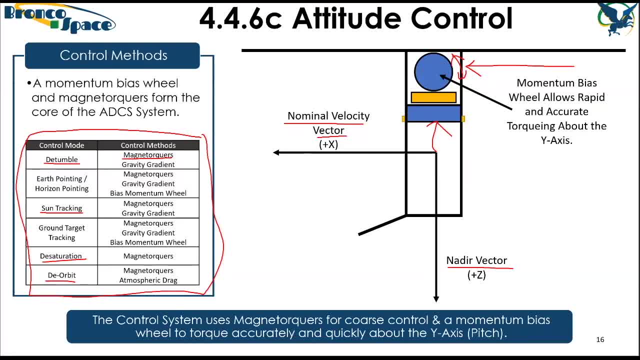 you're going to deorbit on time. But it is good to have some kind of end of life scheme just to keep like space garbage to a minimum once you're done with your mission. And yeah, that kind of concludes like the example portion of the workshop. 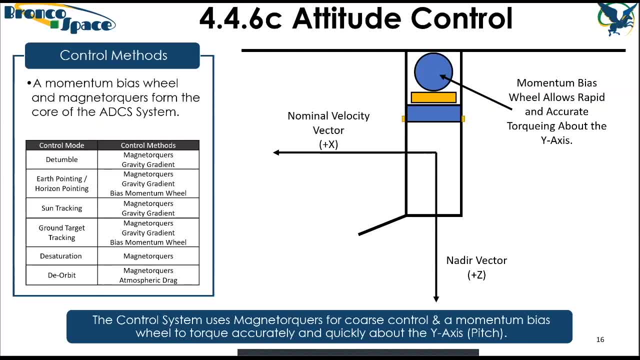 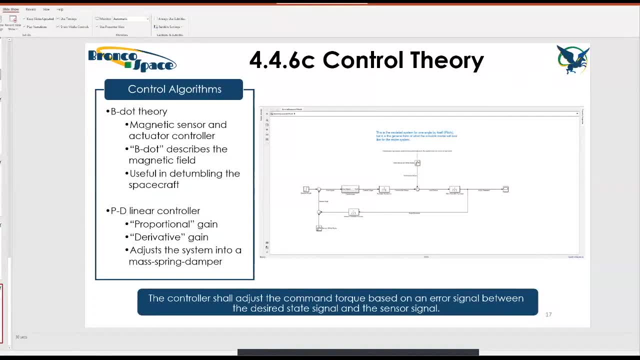 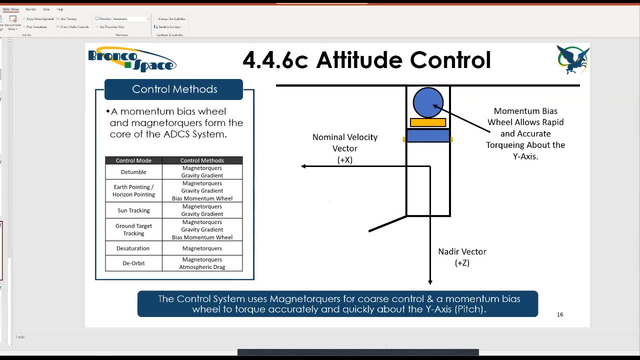 Are there any questions at this point, Like: do I even have anything planned after this? Oops Discard? No, That's pretty much the end. There's a bit of control theory here, right, But yeah, this is pretty much it. 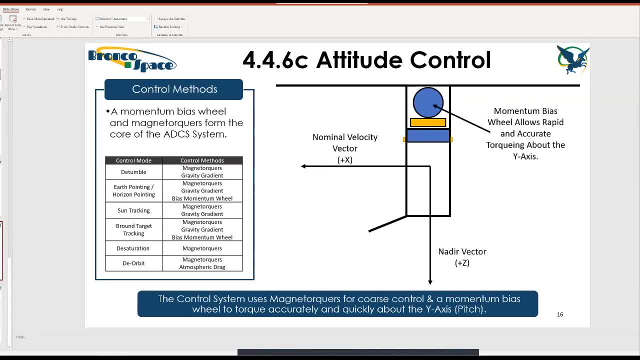 You guys have any questions, you want to bring up Comments. I'd actually like to know if this like made a lot of sense or if it was a little too rambly. It's a lot of content to try and you know. 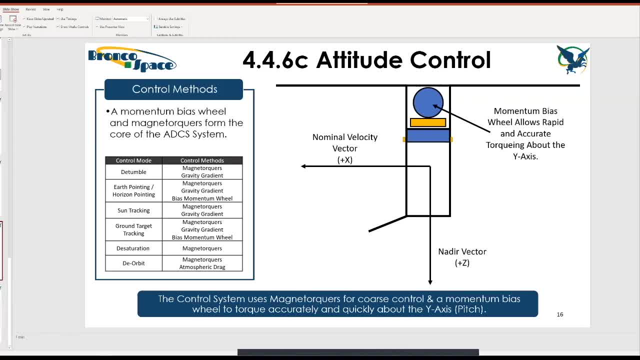 cram in this short amount of time. But yeah, I think we're good, So I'll just stop there And I'll see you guys in the next one. All right, Got one great workshop. That's good enough for me, I guess. 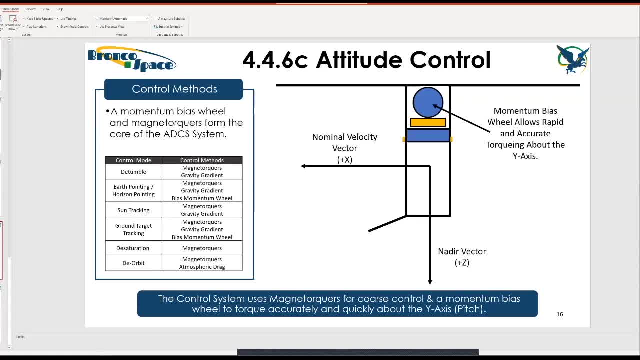